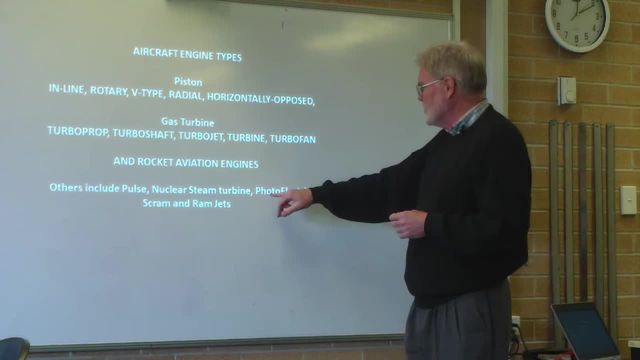 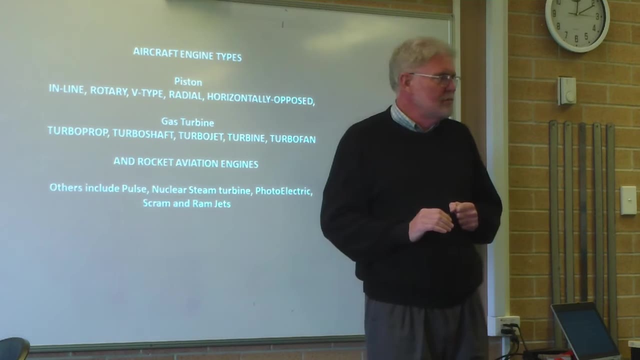 powered engine, right, Steam powered engines- and we'll talk about this in a second- Photoelectric and scram and ram jets. Now, that group of those ones down there, they're slightly novel, They're not your norm. In fact, some of them don't work at all. Some are being tested. 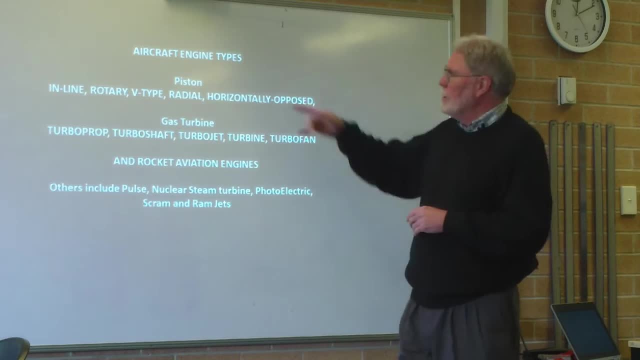 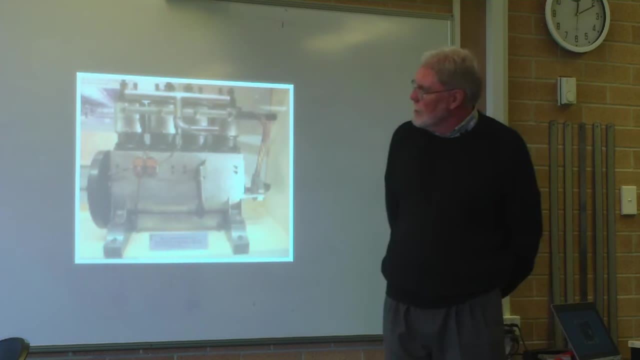 and they haven't got them quite right yet. Okay, so going back to the beginning, the very beginning, it's a good place to start. This particular engine, this one here, is actually one of the Wright brothers' constructions. They had it. 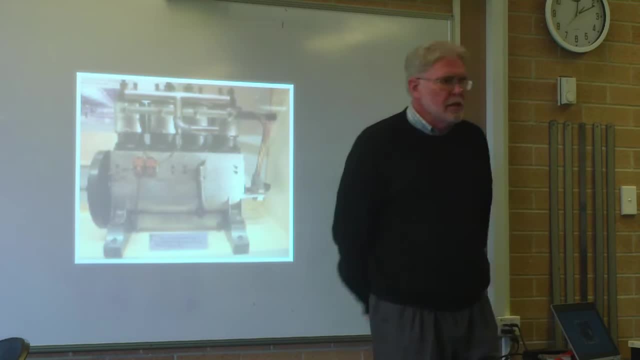 made for their aircraft. Now let's just get the perspective, the time here. So we're at the end of the 1900s. The main mode of power that was being used on large enough scales to be considered industrial was steam. 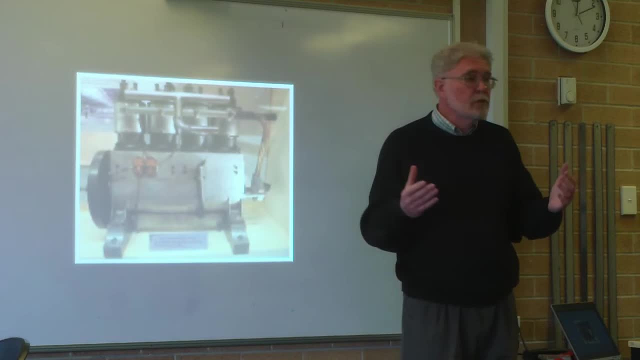 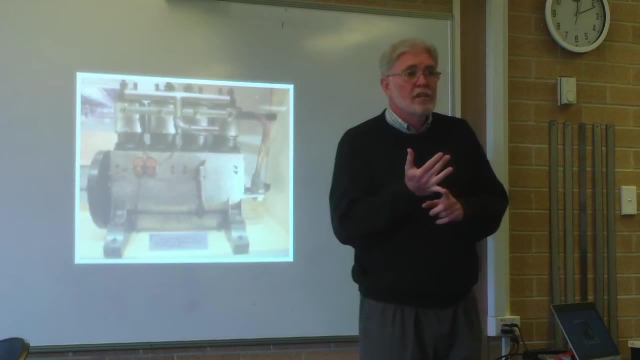 Steam was driving a whole lot of large things. We had steam powered boats, We had steam powered locomotives. We even had steam powered cars. They were not unusual. They are all very large and heavy because steam engines require a big pressure cylinder. Now we get to the area we want to go. into aviation. Big heavy engines do not help you get off the ground. They get in the road getting off the ground. So steam was not the vehicle of first choice. It may have been okay to use heat with a hot air balloon, but then you're lifting a much larger area. It's a bit like a boat. It can take a really big engine because it can displace water to make up for the weight, So it's not worried about it. A steam engine on rails can support the weight, so they can be big things. But when you start thinking about it, think about trying to strap. 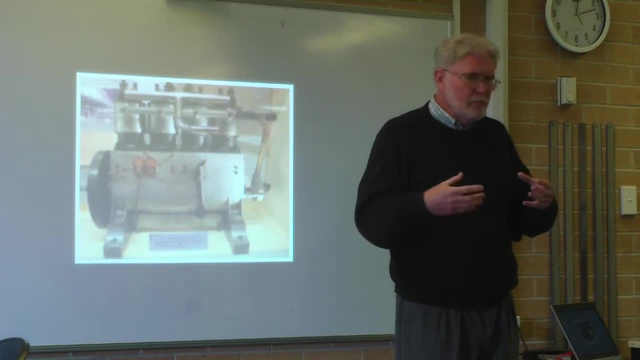 if they don't go very fast, the engines, the steam engines, don't go really quick. Strap wings to a locomotive, It's not going to fly, It's just not going to happen. So it's too heavy. So they had to come up with a small type of engine. And because petroleum was now being 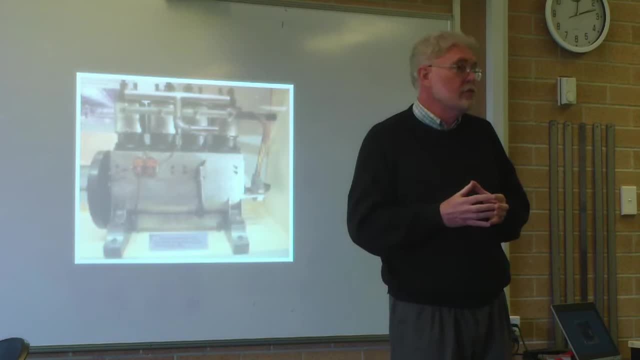 developed petrol engines- internal combustion engines were available- and going into motor vehicles And I mentioned before, first applications tend to be on bicycles And so you get motorbikes becoming a more popular idea because you can make these small motors and they're geared and all that stuff that went into was necessary with 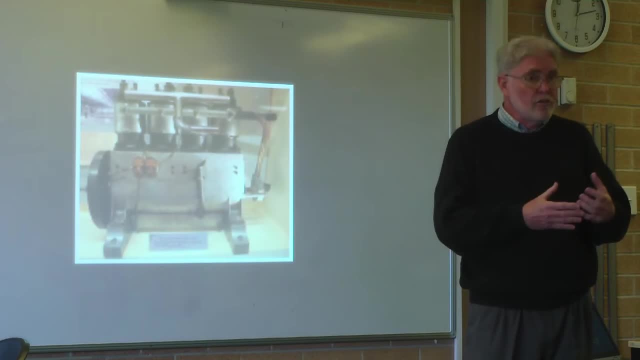 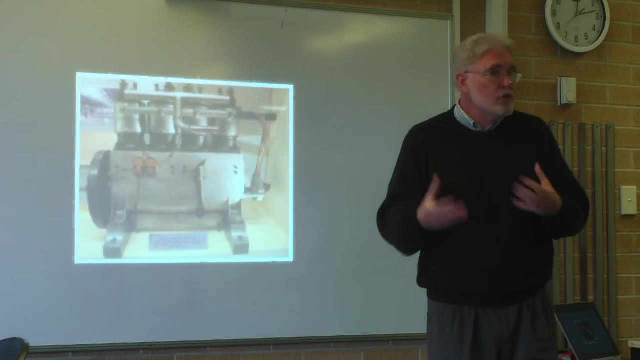 the development of the bicycle helps with the development of aviation And, as I said last time, it's no small wonder that the Wright brothers bicycle repairists were the first people to- well, not first, but one of the first people- to- really seriously look at aviation, because it 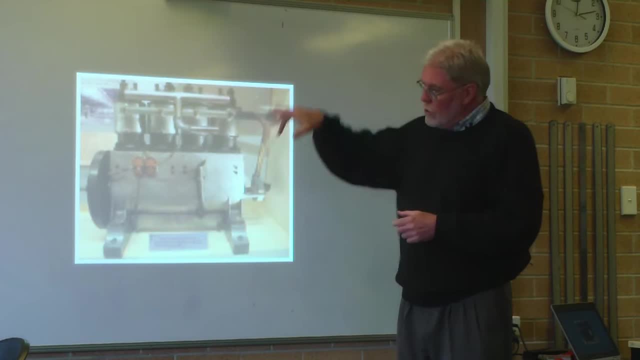 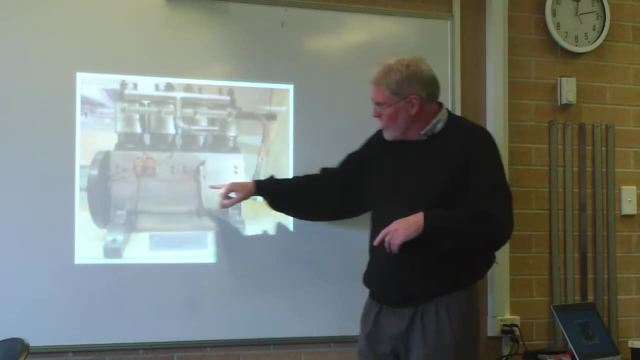 matched what they were doing, So they got this engine. It's a four-stroke, a four-cylinder four-stroke engine. Now engines, as we know from cars, have a long crank case and each of the pistons is operating one. 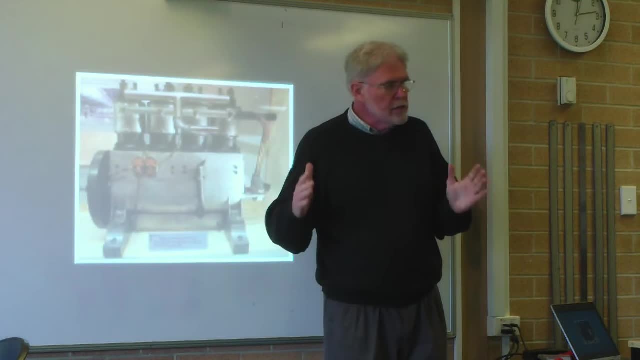 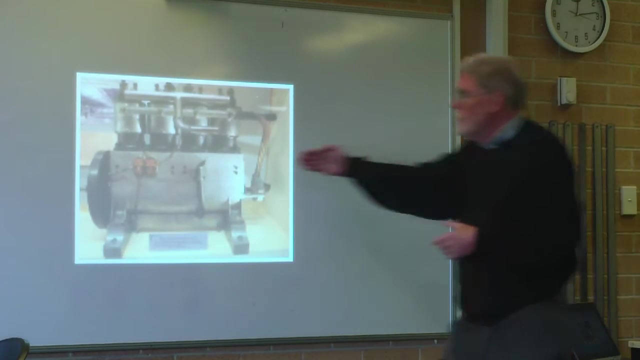 part of the crank and turning it. That long crank case is rather heavy So it works up to a point when you're not trying to go fast and you're not trying to lift a lot of weight. When you get to World War I that type of inline- this is called an inline because all cylinders are. rather slow. They chug away and they have a really large flywheel to keep the consistency of keeping the thing going. So they found that they weren't really producing, one, enough power and two, they were a bit too heavy with that really long crank case and all that other stuff. 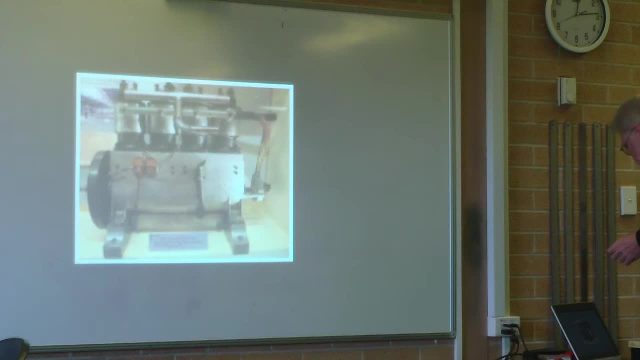 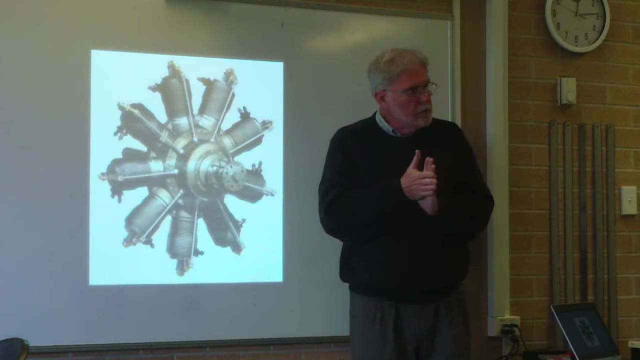 that goes with it. So they started to think about: well, what if we took the cylinders and we put them opposite each other and ran a circular crank rather than a long crank case, with a series of connected pins in this circle so that as each one was going it was rotating the engine? 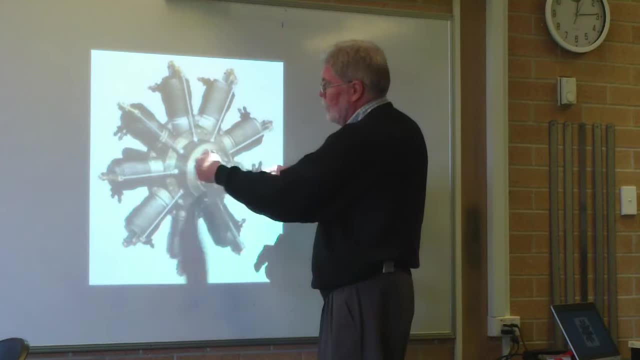 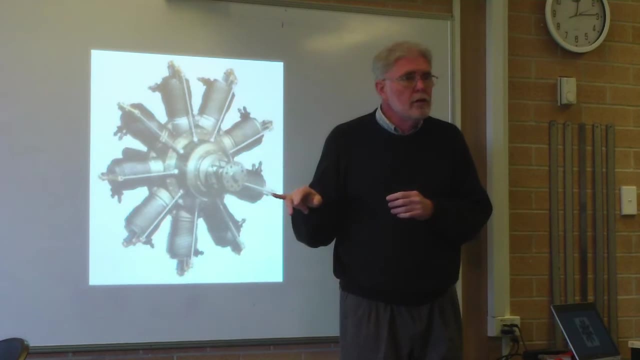 or rotating the big disc and pushing each one as it went around. Not only that, you could now, because you could use the opposite ones that were firing to help drive the whole thing around. you could use them as a compression element, So you can get into a two-stroke situation with these. 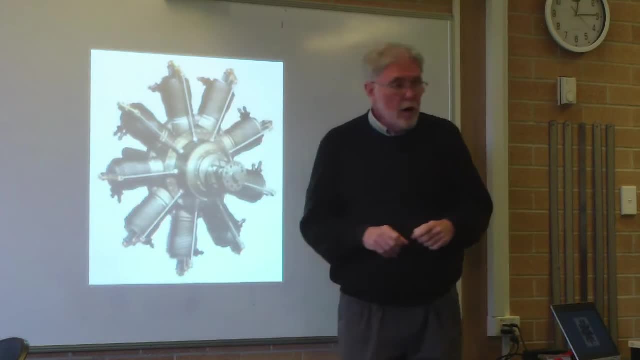 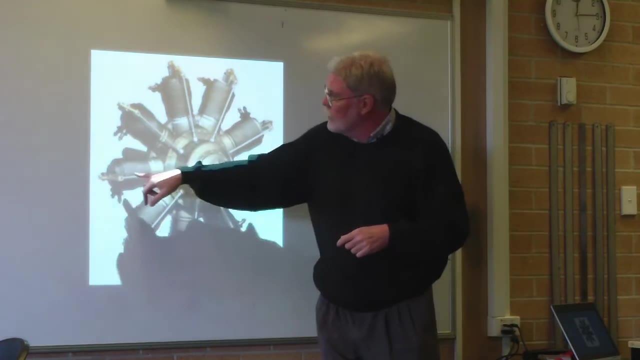 which means that it simplifies all the controls for firing, So you can see the two cylinders. you still had to get fuel in and fuel out, So you still had to have a form of- and you can see this form here- this opening and closing valve system that allows. 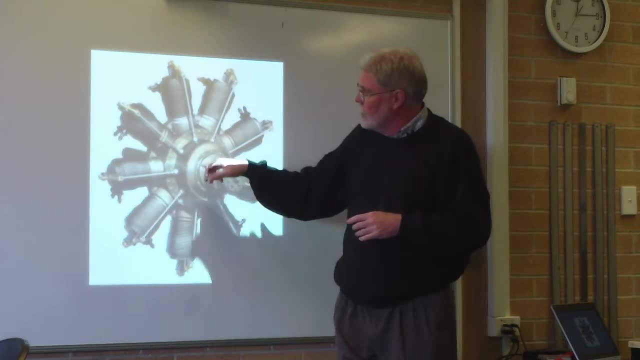 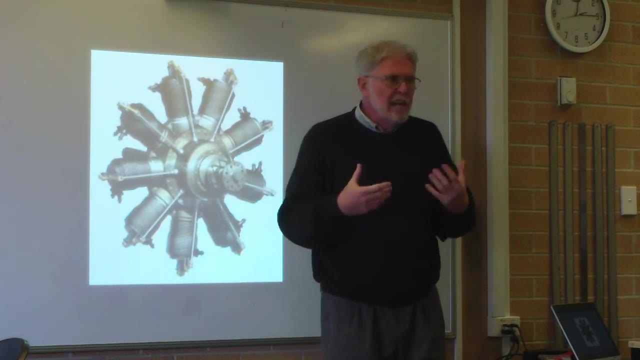 you to get fuel in and out as the cylinders went around. It was attached to a crank in here, so it was timed for the wheels to rotate. Now, the first problem with this stuff is that they generate heat. Your inline engine that we have developed for a car, or for a motorbike, or 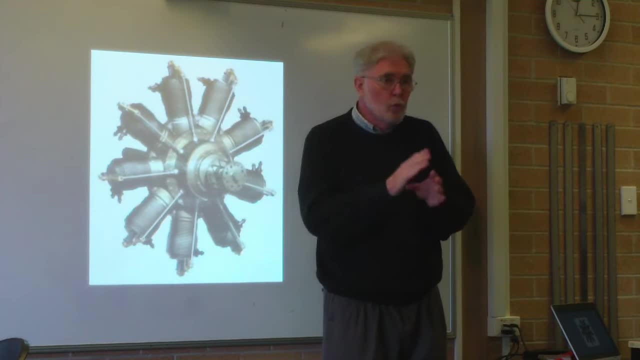 something on the ground could be cooled down So you could have a lot of fuel in there. but it's not going to be cooled by running water over the jacket, water over the engine. Take the water away, put it through a radiator and cool the whole thing down. Now, if you start carrying water up in 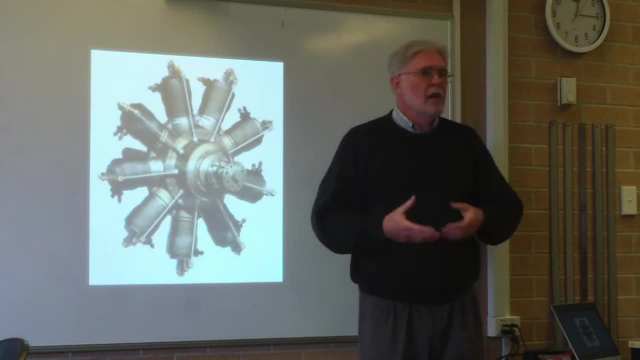 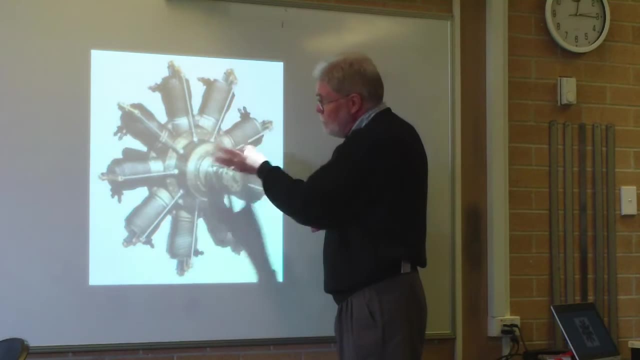 the aircraft. you're now increasing the weight, So again trying to minimise weight. one of the solutions was that we keep the engine open. all the cylinders open have vents. You can just make out the vents around the engines here. air vents, little vents that dissipate heat. so the metal. 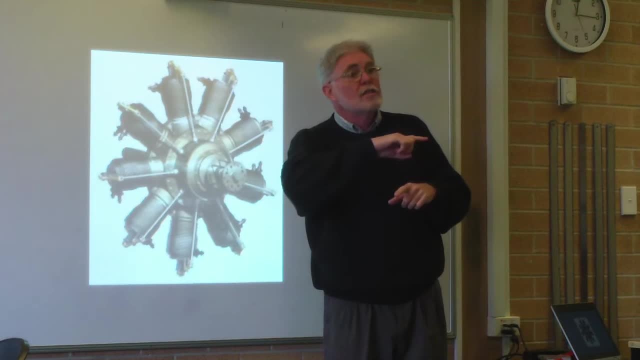 doesn't come up, but it'd have lots of surface area and it would itself spin in the air. So they attached the propeller at the end, They locked the crankcase to the engine. The crankcase itself was locked to the frame of the motor, the frame of the aircraft, and the propeller would spin one way and 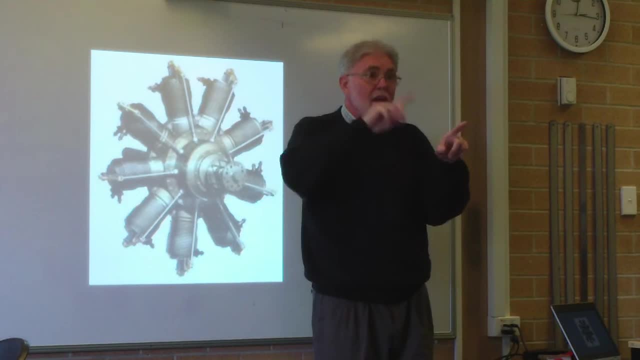 the engine would spin the other And that would cool the engine as it was going. This is called a rotary engine. Now there's a couple of things that are really strange about this process of spinning the engine with the propeller, And that is that it has a lot of torque in doing. 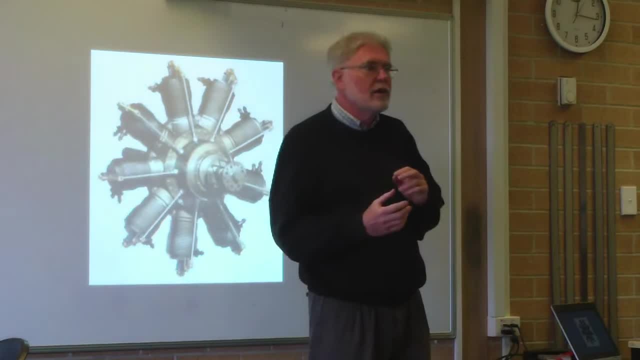 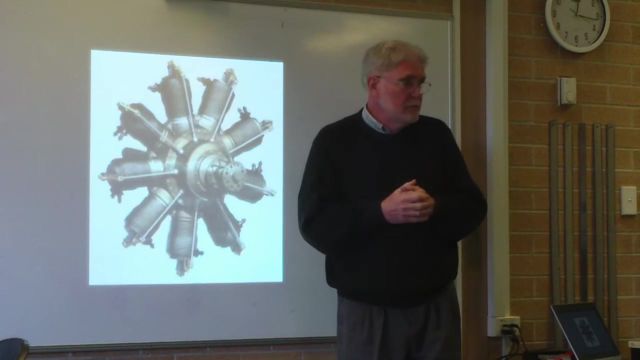 that, And so the engine itself is constantly throwing over. And these planes were extremely dangerous to fly because they wanted themselves to tip over, So you were constantly trying to hold the aircraft from flipping itself. So they were difficult to fly. They were okay up to a point. 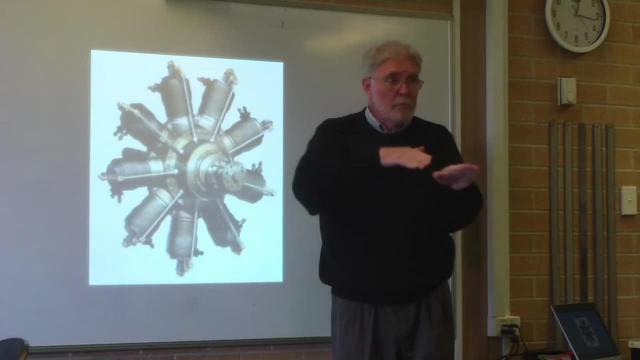 So, as you started to get into dogfights- the situation we talked about, where you know, having an advantage over the other guy by speed and maneuverability- maneuverability being the key thing- that sort of thing got in the road. So they said, well, let's just hold the engine in place. So they went from rotary spinning the 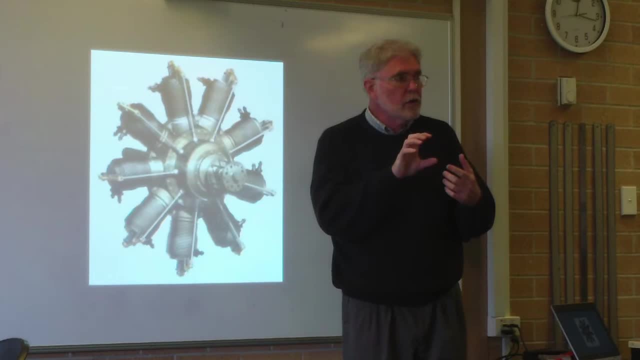 engine, to cool it down, to holding the engine and letting the propeller do the work. Now it still had the propeller weight trying to tip the aircraft over. You may have seen pictures of planes in World War II with dual engines. Well, they did have dual engines in World War I too, but fighter planes with dual engines. 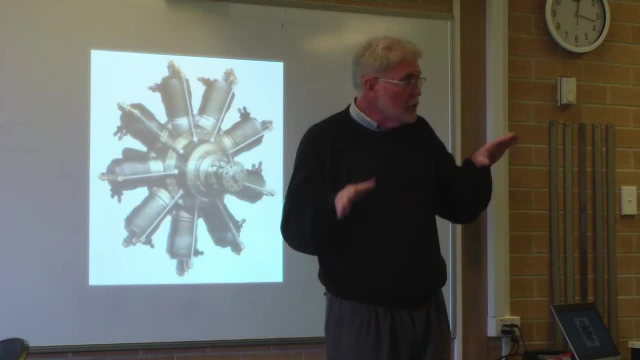 and in those they often got the propellers to run in opposite directions. so the aircraft was more stable. that didn't want to tip over, But any aircraft that any propeller that is going in one direction only is going to want to twist the aircraft. There was another solution which we'll. 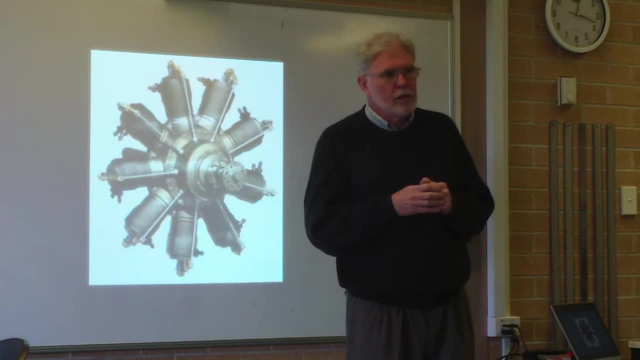 see when we go over to the Air Museum, that some of the aircraft done in the 50s would have a crank case that had two gears on it and one would counter-rotate to the other. So it was. you know, you could just roll the propeller up and it would tip over. You couldn't turn it out, You could you. 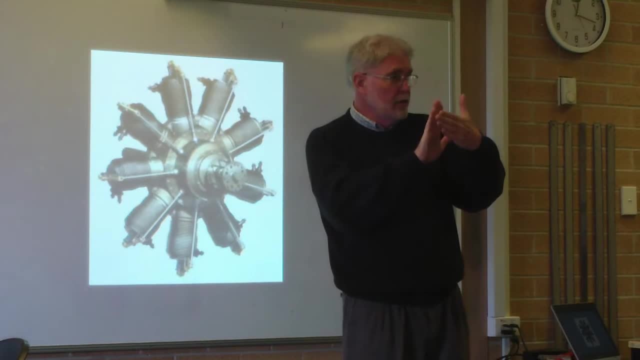 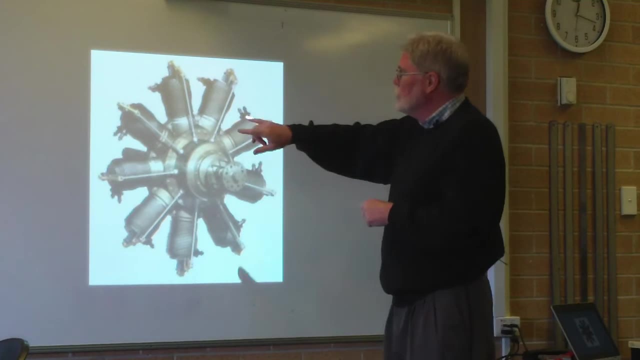 rotate to the other. so they had two sets of propellers, one behind each other, and one set of propellers would go one way and the other would go the other way and that would stop that gyration effect that's happening. and this two groupings, when it, when the motor spun, it was 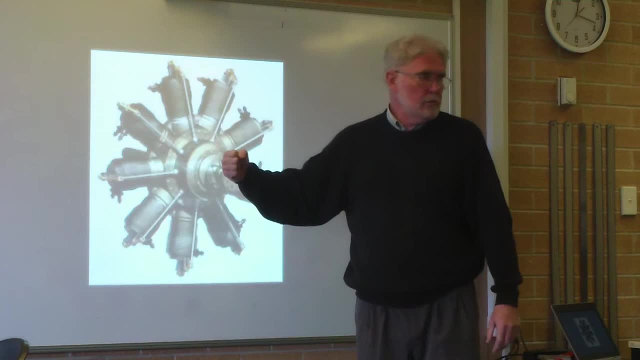 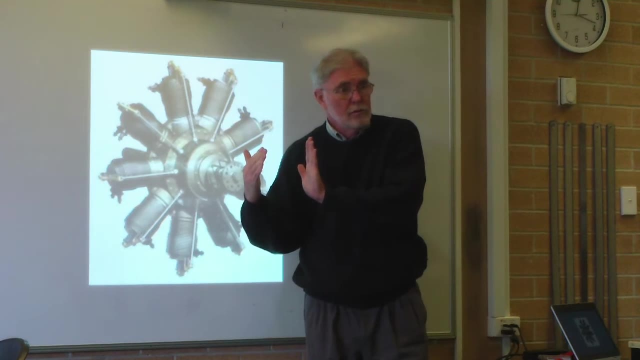 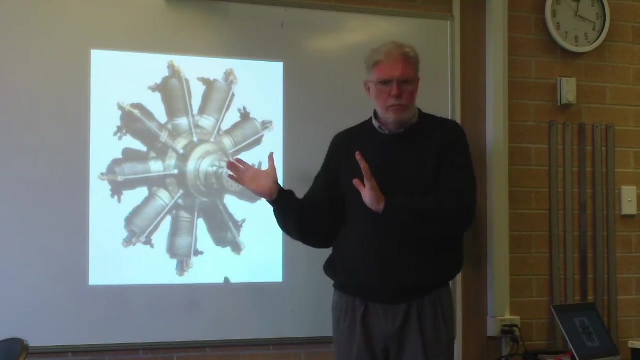 called a rotary and when it was held still, it was called a radial because of the radiating nature. now, the other thing this does is it's smaller, more compact. being smaller makes it lighter, so for a while this was the way to go, so they needed to just let this, probably right through. 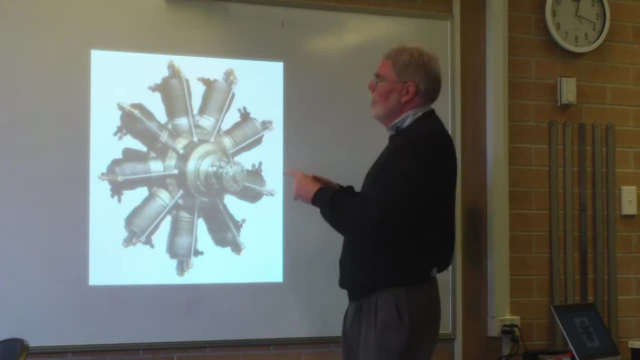 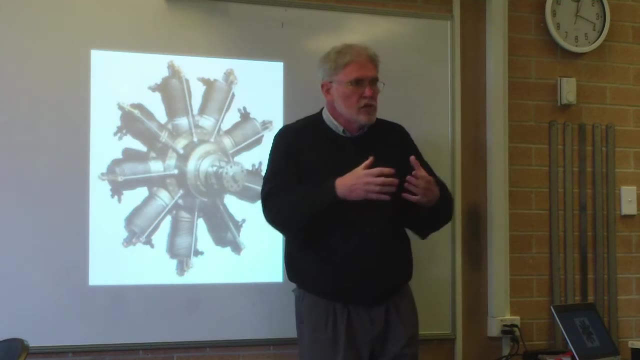 into the 30s and 40s, you'll see pictures of aircraft with um. next thing that happened: to get the airflow over it, they put that big cowling over it so it had a sort of a wrapped over piece of metal that sucked air in and around the engine and outside of the cowling so often on on these. 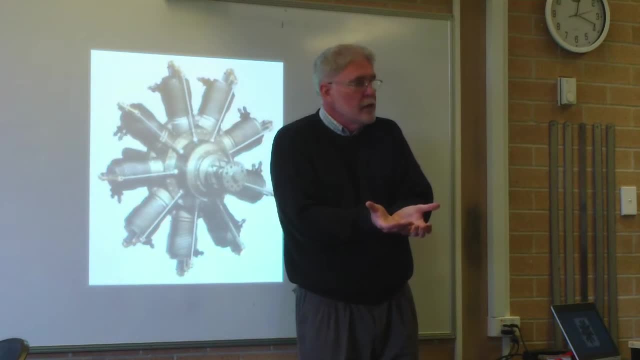 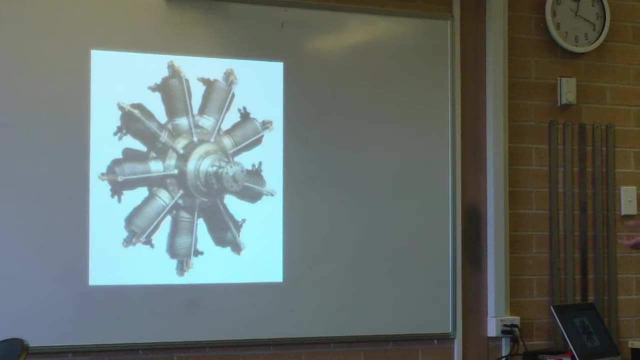 planes. you see this big round piece of metal in front of the engine and then nothing behind it so the air could flow over it and it was actually directing air over the engine. so it was a great way to get the engine to cool it down, because you don't want to be carrying water. 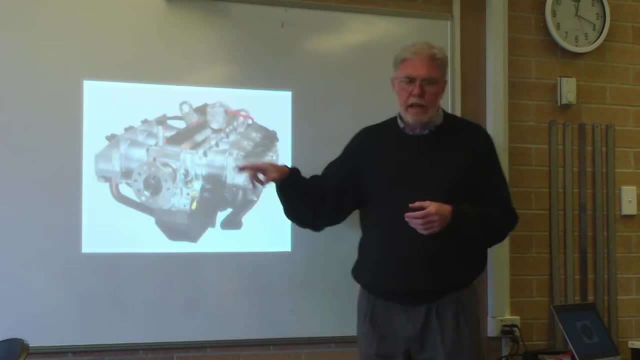 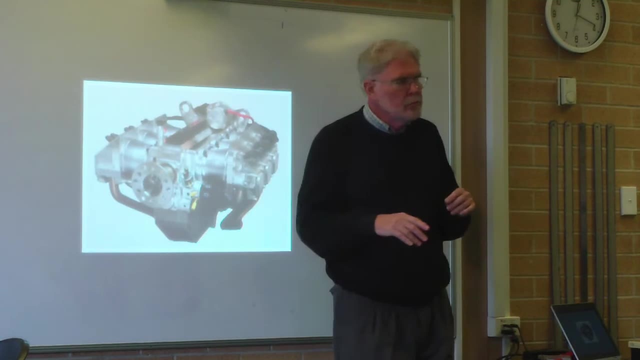 another solution was to have the engine sticking out the side of the aircraft, so it was into the airflow and then you could. you could actually introduce some water cooling. um, but you, because the end, the engines now are getting more powerful, and this is, of course, a flat bed, it's, it's just a 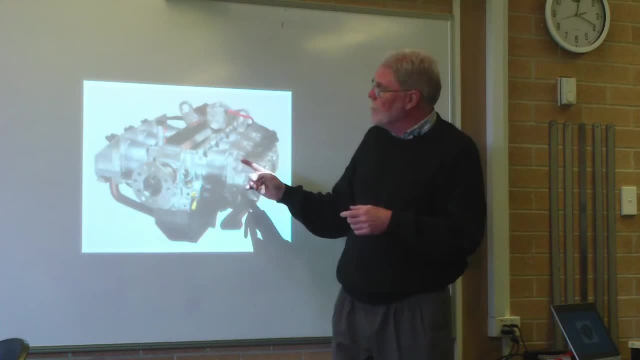 flat line it's. it's like an inline, but instead of having them opposite and having a really long crankcase right. so the the. if you had six cylinders in a in one line, you'd have to have a longer crankcase, and so now you've shortened it down. but you've seen pictures of those, particularly the ones were 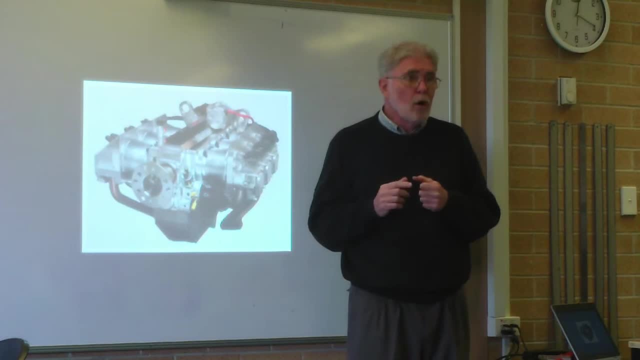 in racing type situations, what i mentioned. you know that pole racing became really important after the war and they moved away from those big radial engines. can you think of a reason why, if you were going into speed racing, you would want to make the engine smaller, in a sense, in terms of 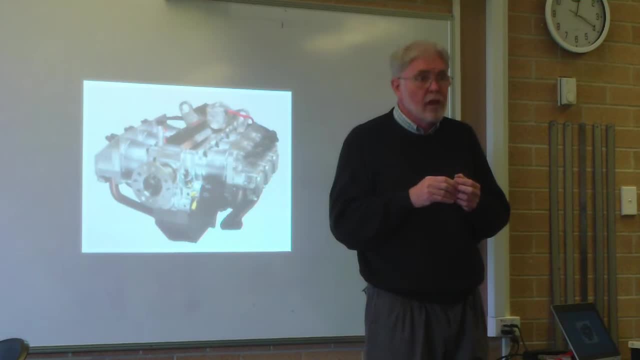 how it hit the air aerodynamics. yeah, so in in see if we can get a picture up here. you can make sense of it. so if you've got a really large round engine at the front with your propeller on it and that the aircraft out the back of that, this is all fronting onto the airflow, all right. but if 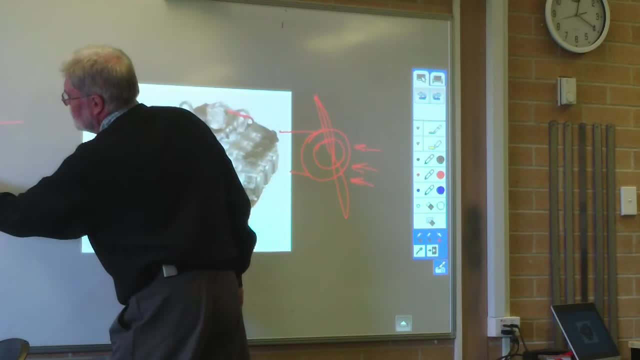 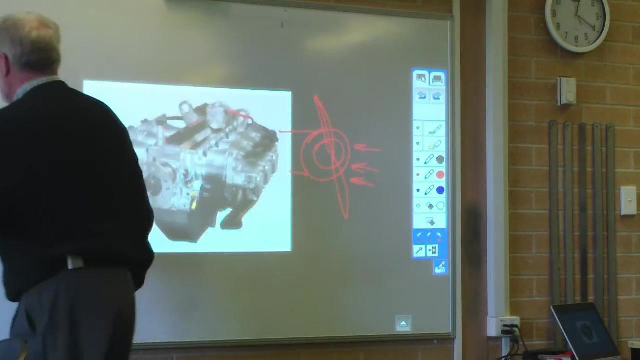 you can make it a flat engine. so now your engine propeller is at the front here and you can have an air scoop underneath and you can have the side of the engine coming out, the side of the aircraft. now you can have cooling as it goes past, air cooling through, as well as a radiator and your 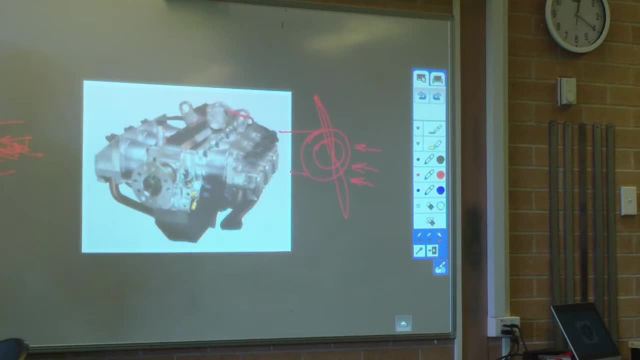 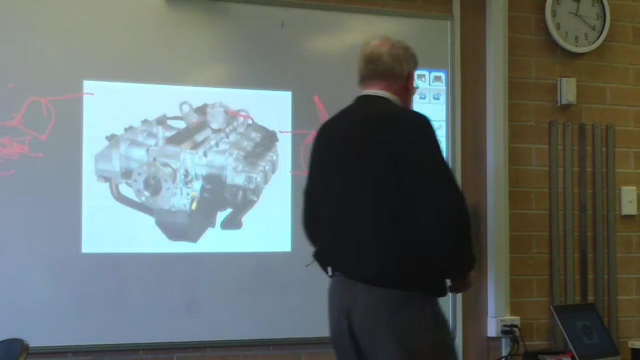 propeller and you can design a much more streamlined looking aircraft, and so that's the beginnings of what you might consider a normal aircraft for maybe world war ii. and remember that the speed racing developed these ideas, and so you had flat engines now if you wanted to get really 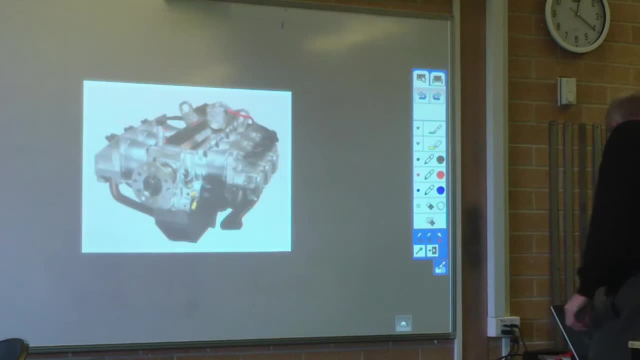 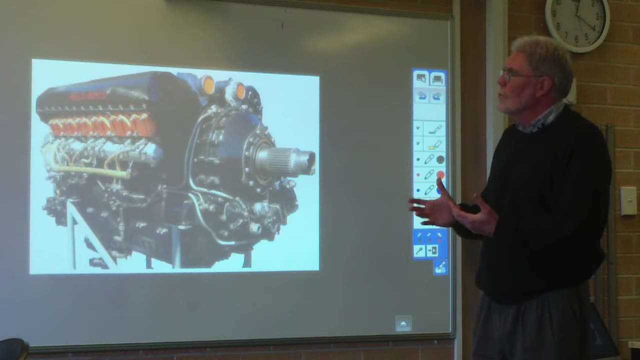 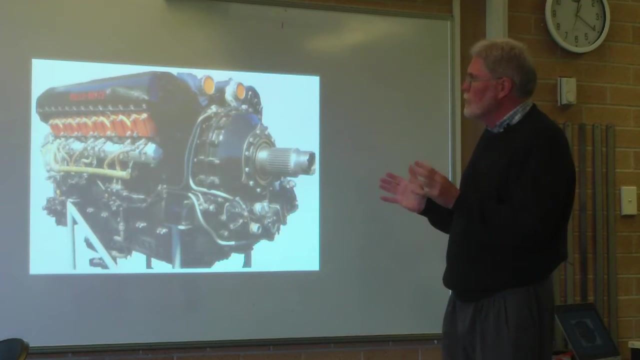 powerful engines, really, really powerful. you just made a brute of an engine, all right, and this is the famous rolls-royce merlin v12 engine and basically it's everything you know about normal engines. it's it's actually, it's got things going on it like it's water cooled. it's normally. 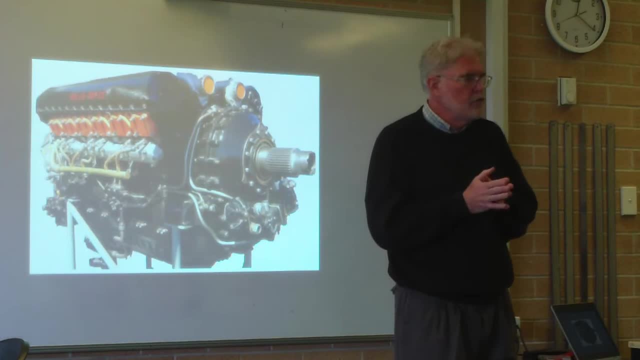 aspirated, which means it's in a carburetor with injectors that get the fuel acid spread. so it's a small engine and the engine doesn't just go back and forth. it's a kind of a electric engine. it's got a lot of different things going on. it's got six cylinders on each side, so it's got a. 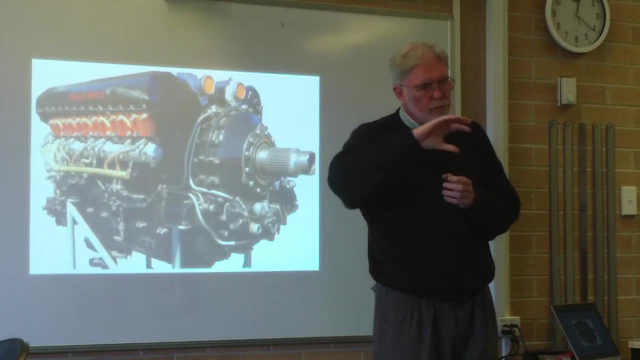 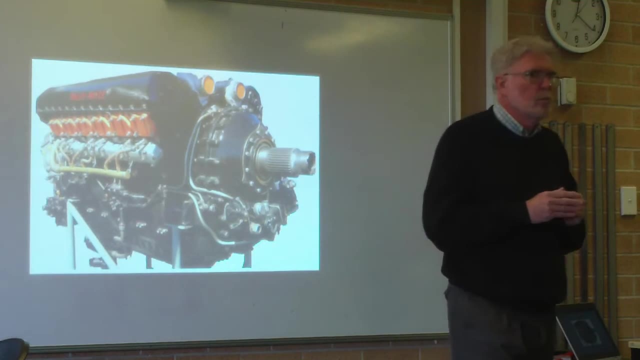 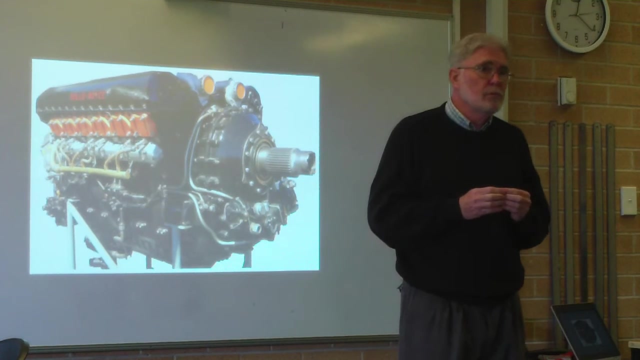 fan forced for driving, that drives a fan at the back which supercharges the engine, pushes the fuel in and spreads it out better, so it burns at a higher rate and gets more power. and this is the kind of engine that was shoved into planes like um the spitfire. you know, these big engines rolls. 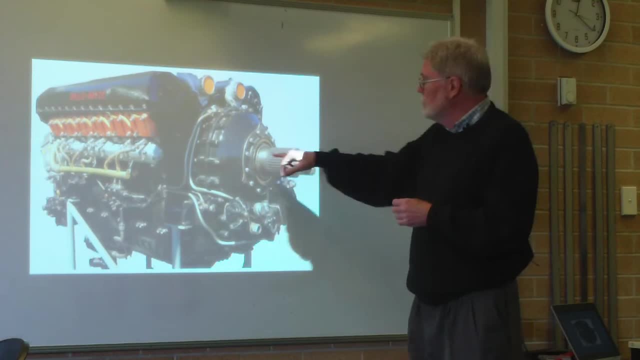 royce merlins um single engine engine. you know, sometimes it's the most powerful engine ever. and single engine engine, you know, sometimes it's the most powerful engine ever. and single engine engine drive shaft. still so ran one propeller out through the front of the aircraft. 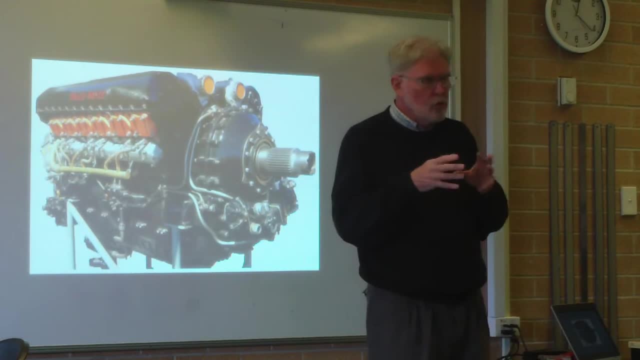 Now, very briefly on propellers. now I said we'll talk about them as well. the idea of an air screw or air propeller as an air screw, is that it grabs the air in front of you and drags you through it. It also by virtue of going really fast. 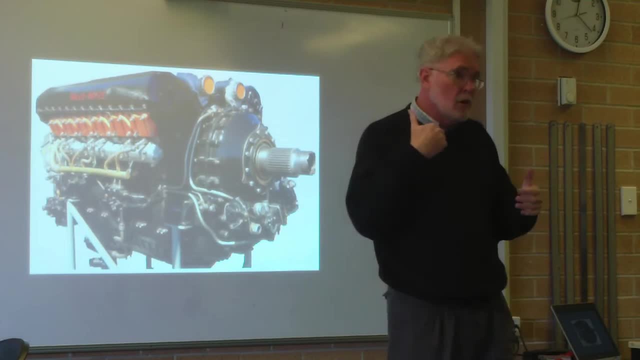 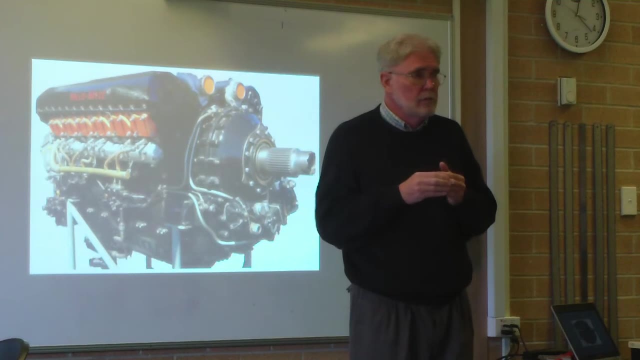 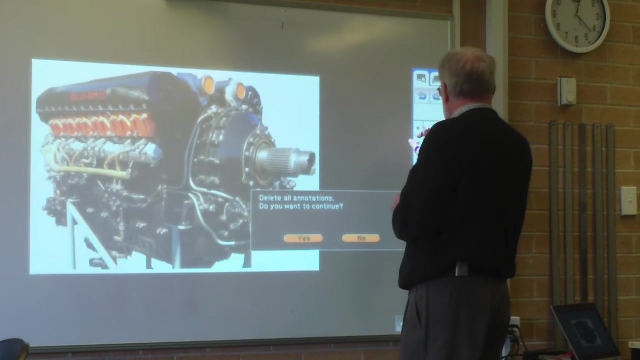 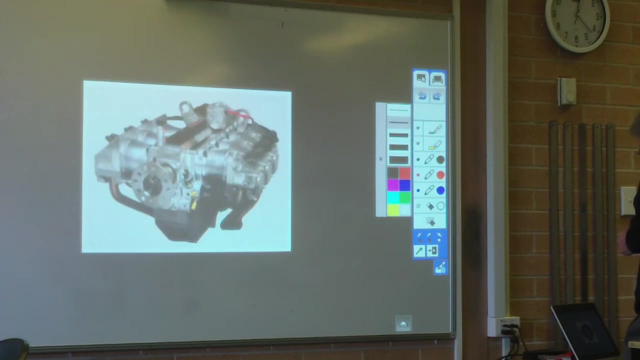 generates a lift in front which pushes the air behind you and gives you a thrust situation. So, propellers, you have a limit to them, though clearly, one of the limits is going to be- I'll use a different colour- something a little bit brighter, a bit more area on this one- if you have an aircraft on the ground, just a normal aircraft, and your propellers are here. your size of the propeller is limited to when the plane is up and running to take off, simply because if you don't watch out, the propeller is going to hit the 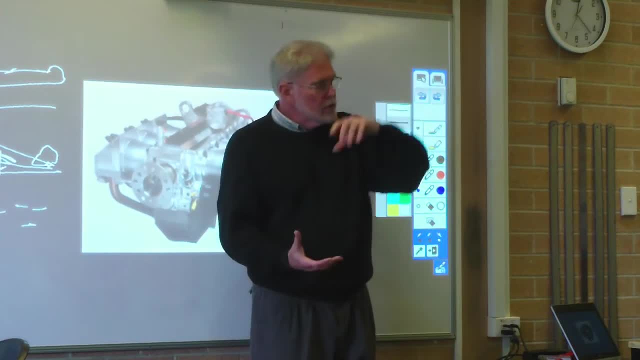 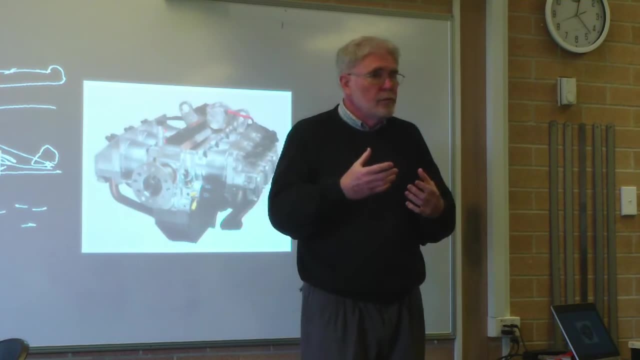 ground. So you've got a limitation on the size of the propeller. Now how much air you can grab is going to be related to the size of the propeller. So one of the options you can do is to increase the number of blades on the propeller. But then you start to get to a place where you actually get one blade getting in the road to the airflow of the other. So there's a maximum five. six is probably about as high as you're going to get, because then the space between the propellers isn't enough to drive enough air. So you start to cut into yourself a bit. 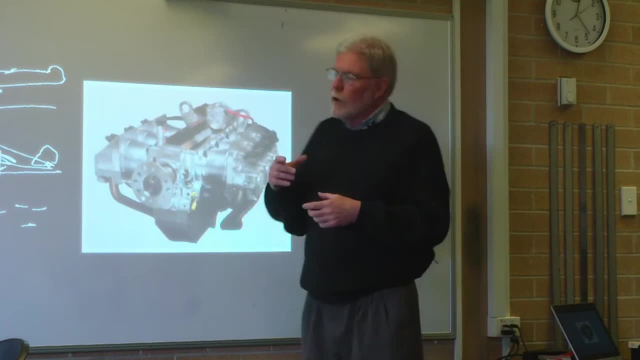 So propellers are an interesting thing. If you go really fast you can make them smaller. Some of the designs of propellers now are such that the outermost point is the fastest point on the propeller because it's the largest circumference. it's spinning the fastest, So you've got to worry about tip speed If you go too fast. 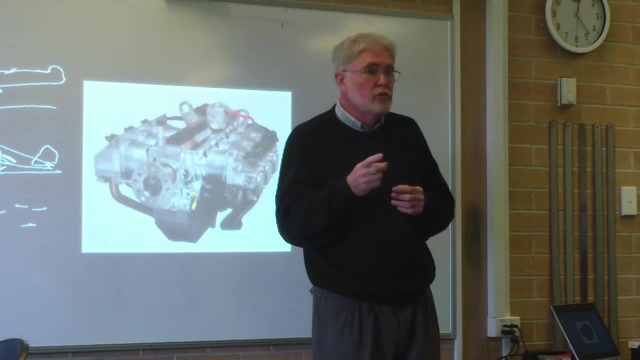 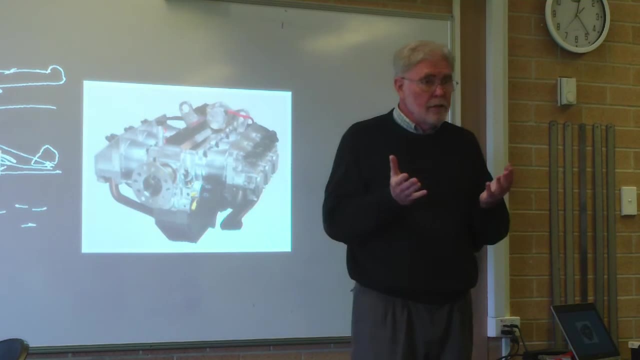 on the engine, the tip speed of the blade might be sufficient to have it disintegrate itself, So it'll fall apart, particularly if you're making a laminated wooden blade. So you might want to try doing all sorts of different designs, And so they did the design. 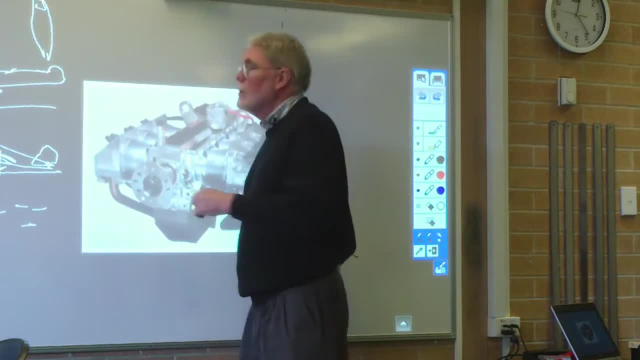 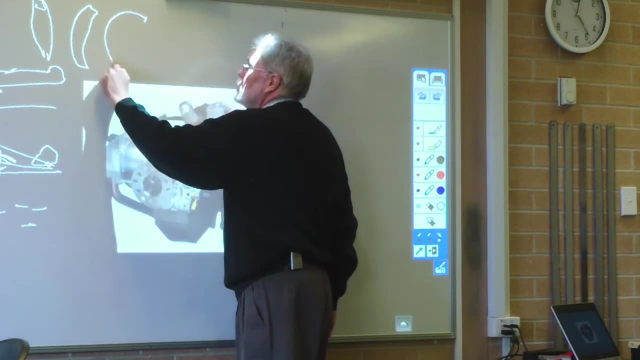 so that the edge of the blade at the end might have a metal tip on it. Another one that comes out later is they actually bend the blade, And the one that's the worst looking is the sickle blade. So the propeller is actually like a series of sickles that bite through the air, And that's so. 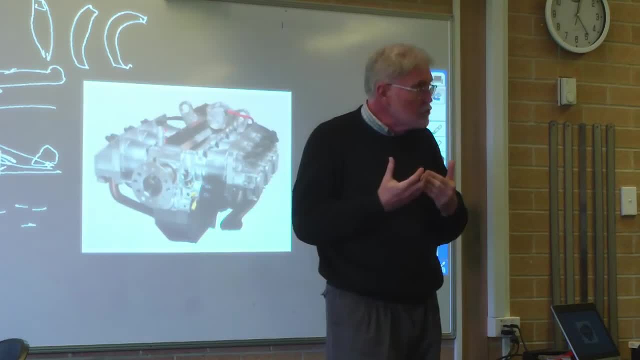 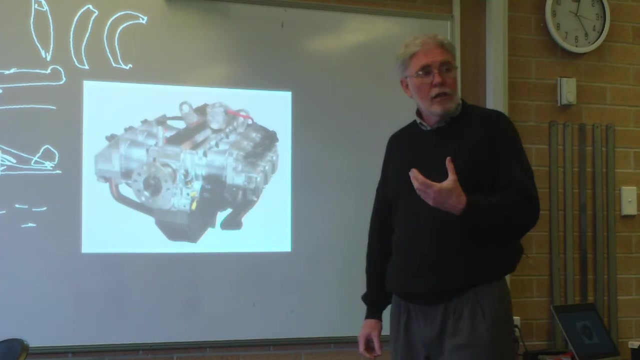 that tip speed there, maximum amount of air being pushed back and without the tip speed. So you want small diameters if you can manage, And so propeller design becomes a really interesting property, combining propeller with the engine capacity And if the engine's not powerful enough, putting a big propeller on. it's actually going to. 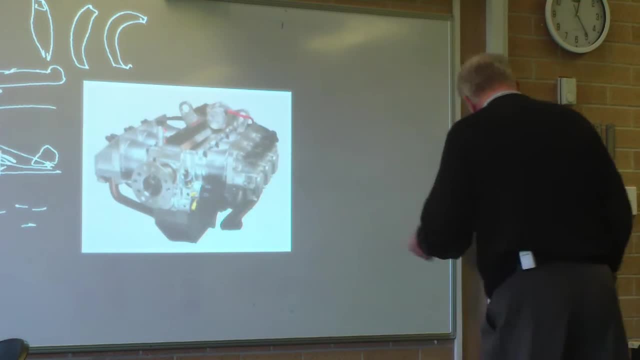 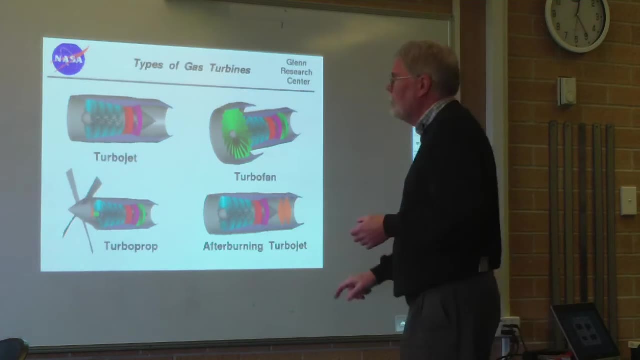 detract from what you can get out of the engine. It's got to be able to drive it, So let's go back to our next one. All right, get rid of this. So there's your propeller piston petrol engines Now. 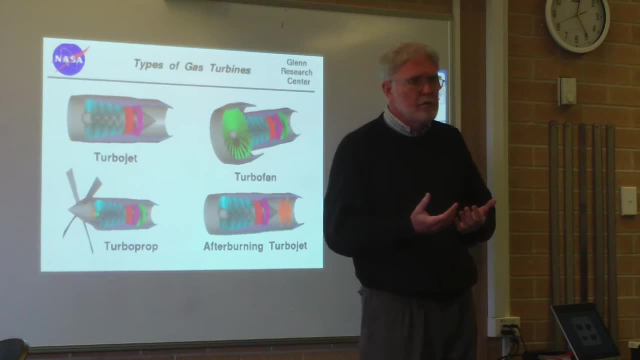 the propeller piston. petrol engines are pretty much run on some form of fuel. Aviation fuel tends to be a lot finer, and finer in the sense that it's more refined, So it has a higher octane. Because if you're going to carry something with you into, that's going to be weighty and you're going to have problems with you know flight. if you've got heavyweight, you want to get the maximum out of it, which makes it more expensive to produce, And a lot of early planes didn't run on what we would call petroleum but ran on things like kerosene style. 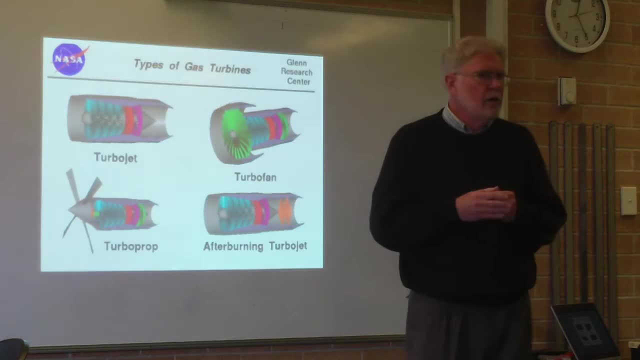 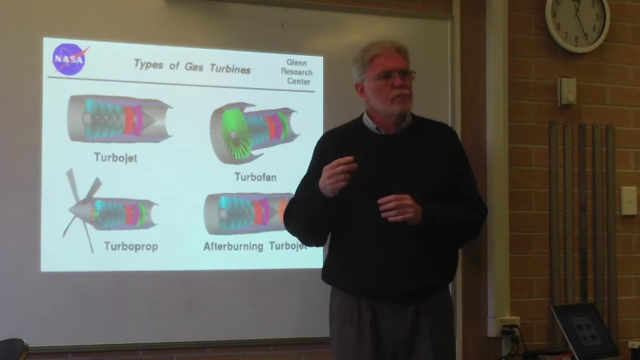 Really thin, high burning fuels with high octane. Later on we changed. let's just step back a bit. Mid 30s there was a move towards going back to a concept that was acceptable from steam engines. When you put a steam engine together, you're really blowing hot steam over a fan. that will. 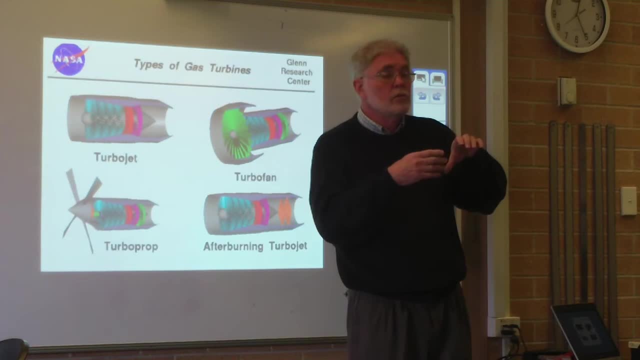 drive a turbine, And that was not a good idea. That was well known, And they used that to generate electricity. That was the common way of generating through a turbine engine. It's just the same as if you poured water down from a mountain, like they do with the hydroelectric schemes which run water over. 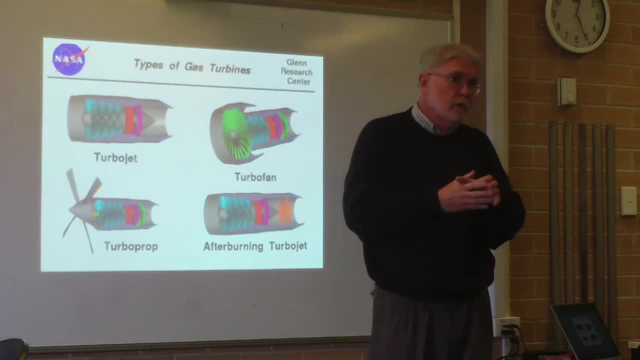 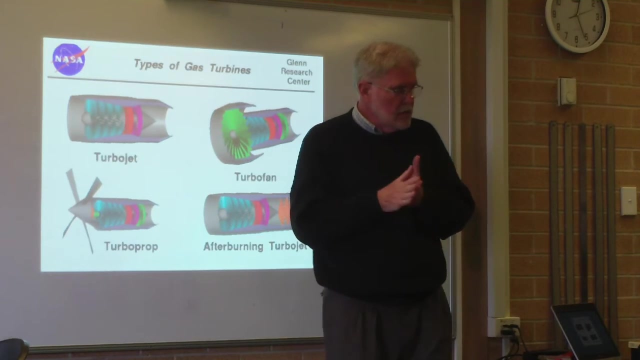 a propeller, An impeller. it drives the generator. So there was an awareness that you can get quite efficient in the fact that you use a turbine. Problem was how do you keep it running once you get it going and the sorts of speed you need to get up to to do it. 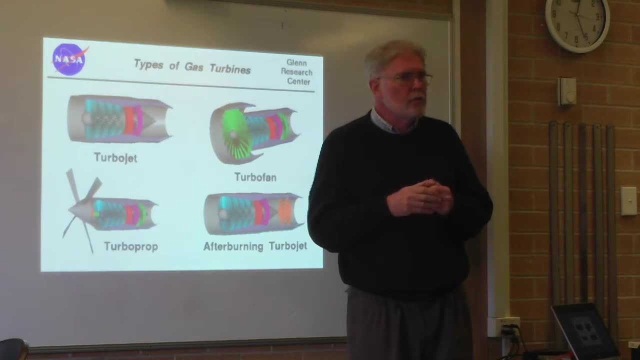 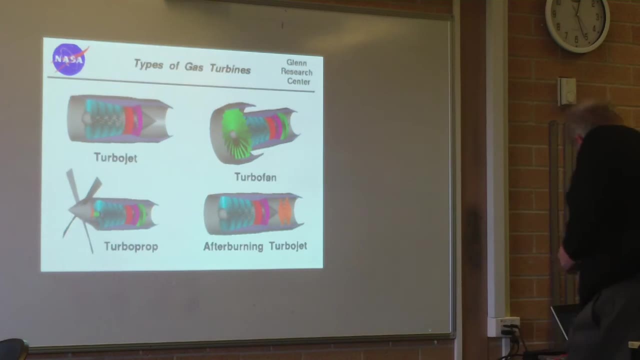 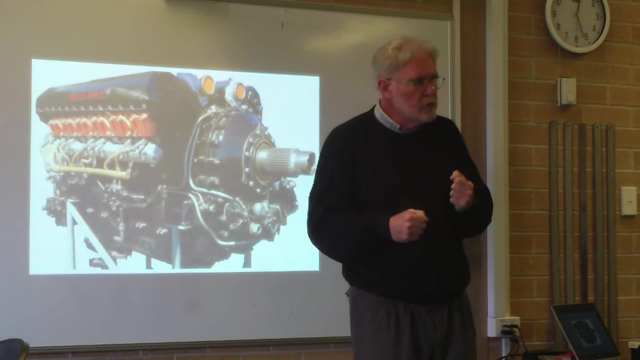 The beauty of a jet engine is it's very, very limited in parts. There's not many parts to it. It's really quite a simple engine. You go back and have a look again at the size of that thing, with all of this cabling and wiring, the time, the cylinders, the big piston rods that are. 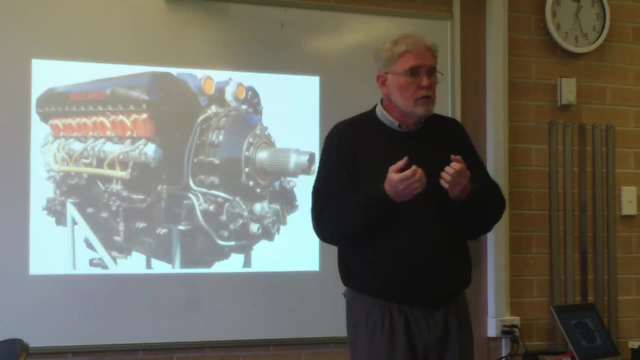 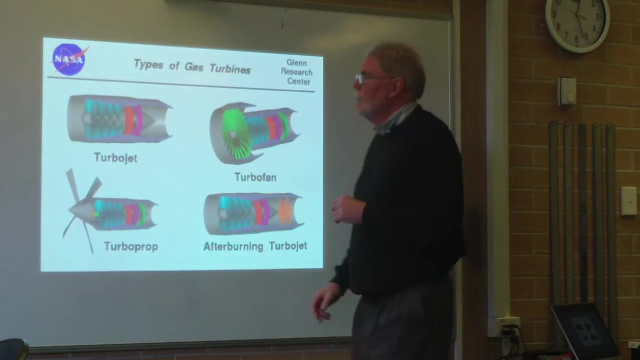 active, Some of it's actually acting against itself. So you're not very efficient because half the stroke is not actually driving. But with a propeller-driven turbine there's constants to it. It's simpler. It's really just a matter of this simple design. What you're doing here is in the front four, or 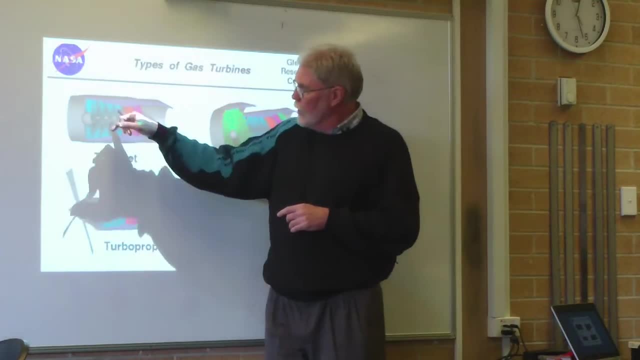 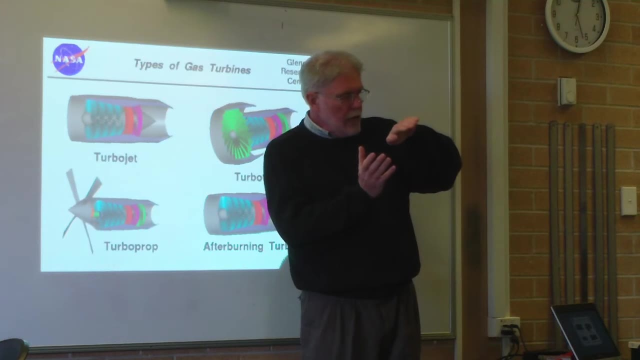 five blades. this is your basic jet engine front. four or five blades. each one is slightly smaller than the one in front and each one tilted slightly differently into the air and it's dragging air from in front and squeezing it, And so it's a little bit of a problem. But with a propeller-driven turbine there's 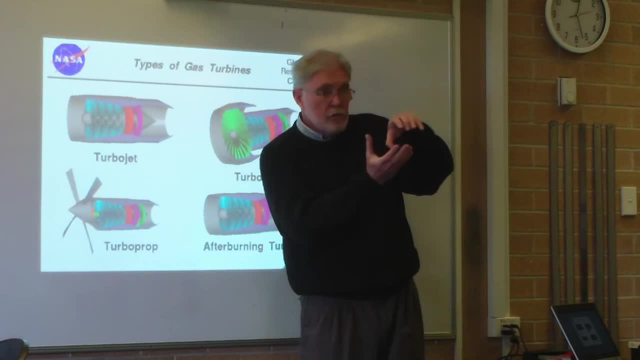 a little bit of a problem. But with a propeller-driven turbine there's a little bit of a problem And pushing it through and speeding it up at the same time because it's got to move through a small area. Remember the idea we looked at with Bellini principle that if 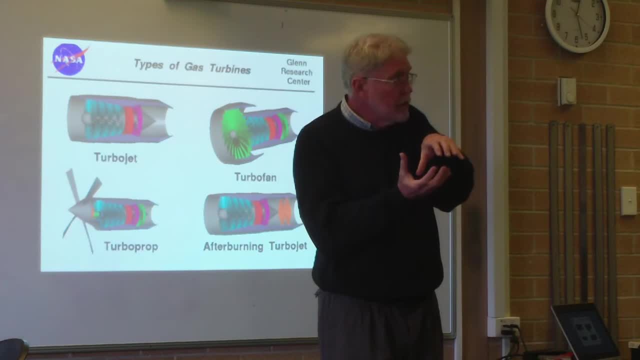 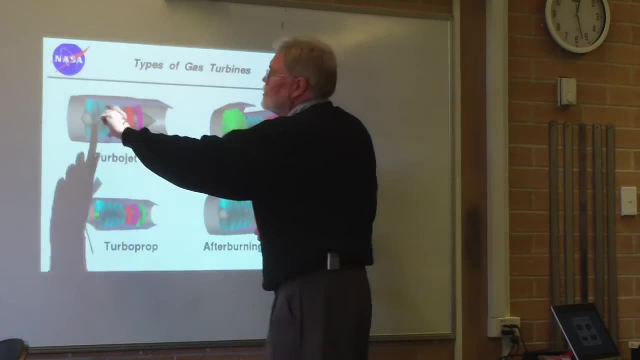 you're going to take the same amount of air into the front, put it out the back. you've got to make it go faster so it doesn't bank up. Otherwise, all you're doing here is creating an air screen in front of you, So it's squeezing the air. Now, when the air squeezes into a 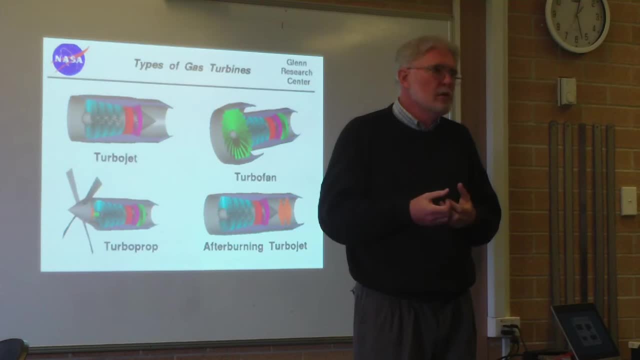 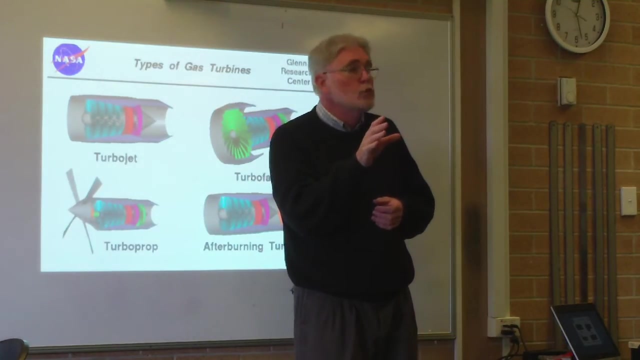 small area and accelerates the level of friction goes up between the molecules as they get pushed through the surface, So it also heats up As it gets hotter. the next thing you do with it is you actually throw some light fuel into it, a small amount of jet, say something. 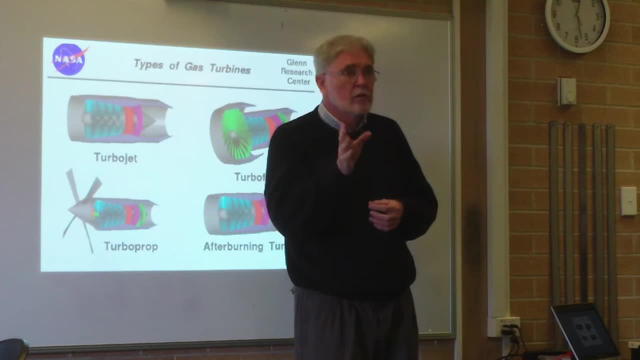 like kerosene or jet fuel, which is a high-octane aviation fuel, and you light it And what that finishes up doing is now heats the air and tries to make it expand, But you haven't got anywhere to expand. You can only keep going. 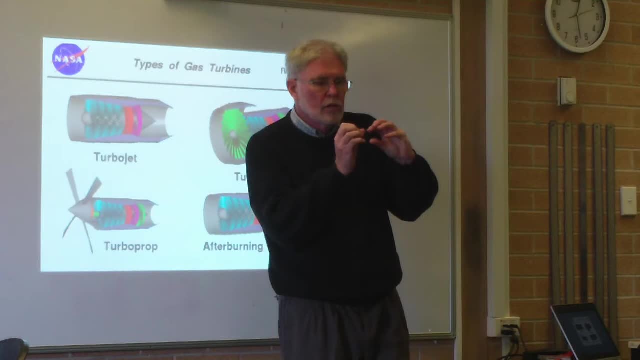 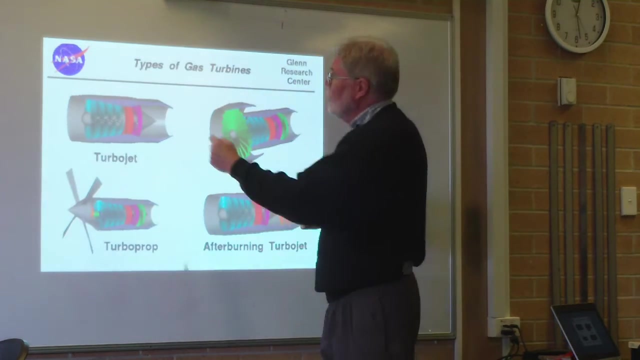 You've been pushed in, so you've compressed the air. and then you get some of that compressed air and you use it to keep a fire going, burning a little fire going inside the cylinder, and it heats the air. The air then tries to expand And as it's going out the back, trying to 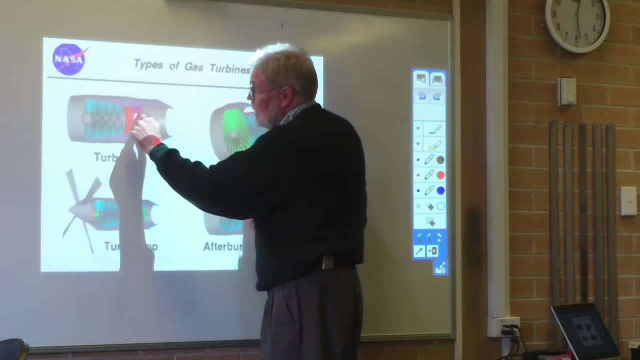 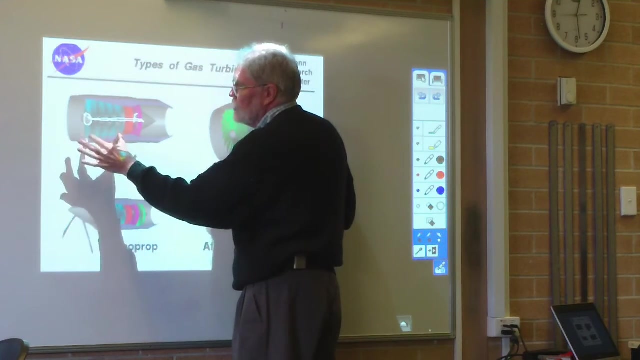 get away. you drive another propeller just in here that is connected to a shaft that runs back to the front, which drives the impeller. So there are three sections to the engine: This section here which is where the compression takes place, Then this part here where the ignition of some fuel sprayed into a little. 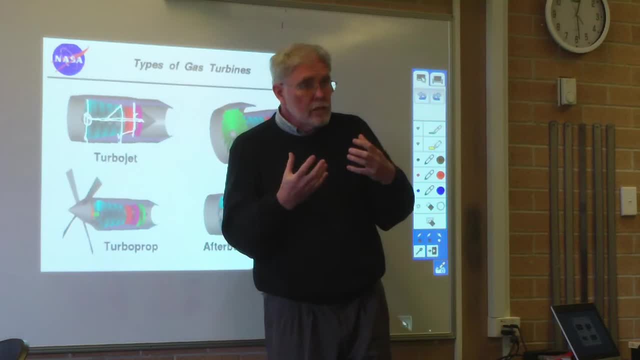 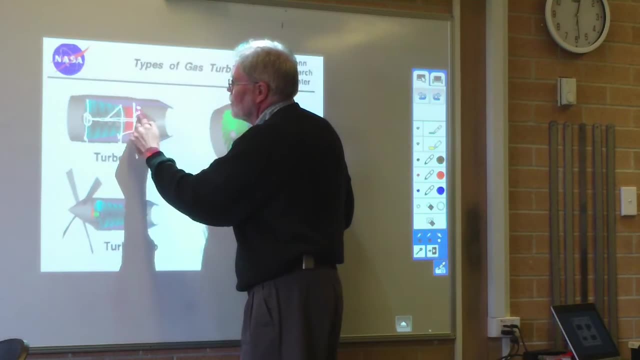 part, a little burning cylinder in there that heats the air up, increases the expansion of the air. so it wants to keep moving faster to get out And it drives a final little propeller at the back which is actually driving the front. 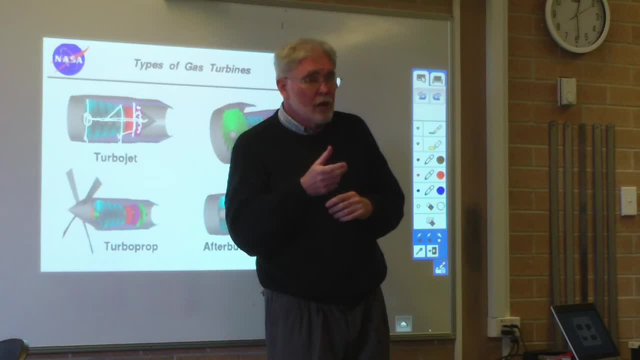 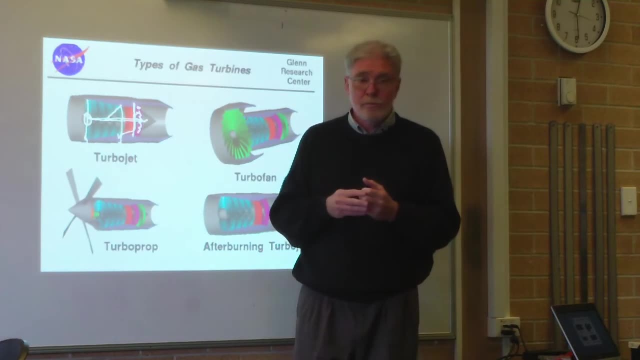 Now the thing is to get it started. You just get the engine going. Now they can do that with other methods. now They have starter engines for it and such. Yeah, just go and open the door for him. So lots of things like that. 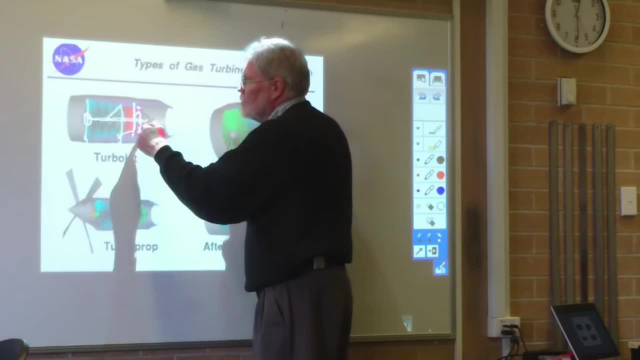 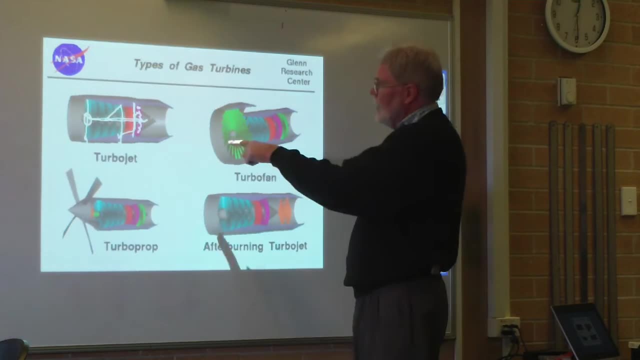 Where am I going? Yeah, So it's really only three parts. One single part through the middle. Once you get it going, it'll run itself, Runs itself. Now the other types here are just all that one single jet engine. 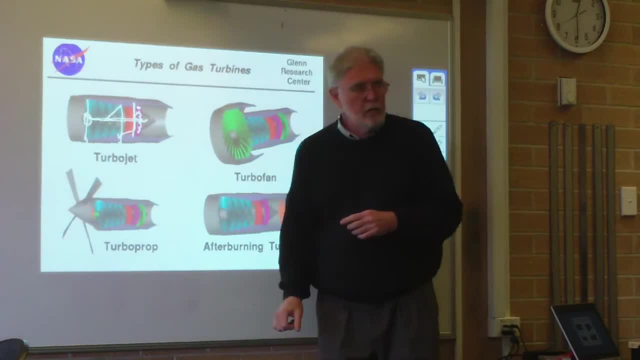 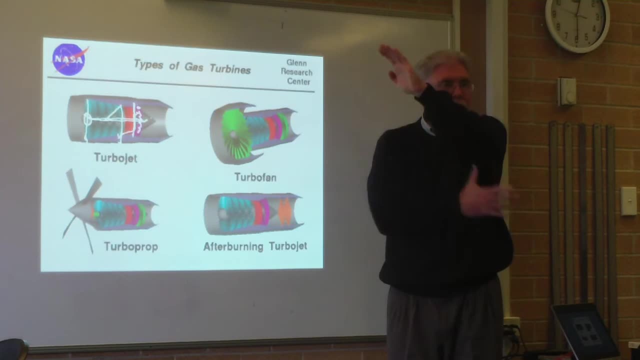 Yeah, That's the engine being adapted to several different types. This one here, the afterburner one, is the one you see on the military jets, You know, the ones that you see flying up with a big burnout at the back. So it's actually going. I'm burning air in here, but I've also 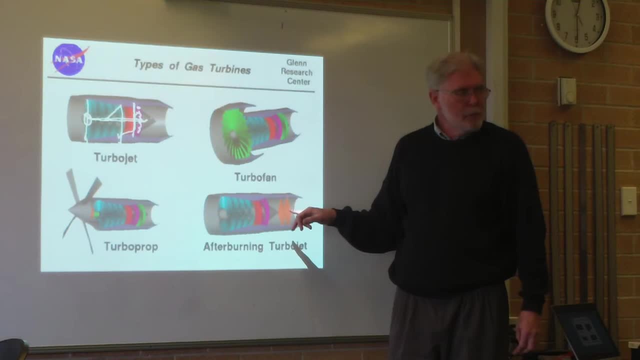 got now hot exhaust gases coming out, Why don't I put a secondary burn at the back, which will even increase it even further? Now, clearly, you're going to burn a lot of fuel when you do that, So you have to be like a military jet where cost isn't important. 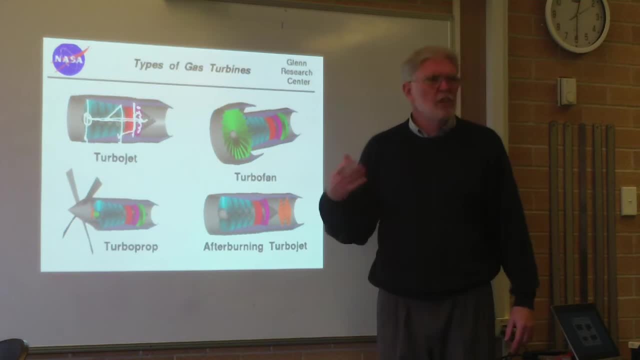 What's important is giving yourself a boost. You don't do it all the time. You only do it in climbing or trying to make invasive maneuvers. So that's where that comes in This type of one we're going to talk about a little bit more in a moment, because it is 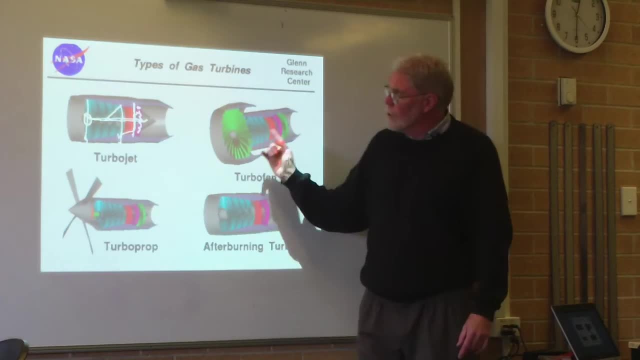 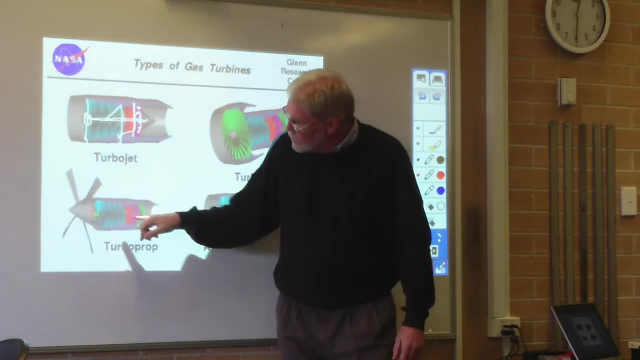 really important And in fact, those two are the most common of the jets we use today on commercial aircraft. And this one, basically, what this is? it looks like a hybrid, doesn't it? It looks like it's got two things going. What's the propeller? Well, you know, I said 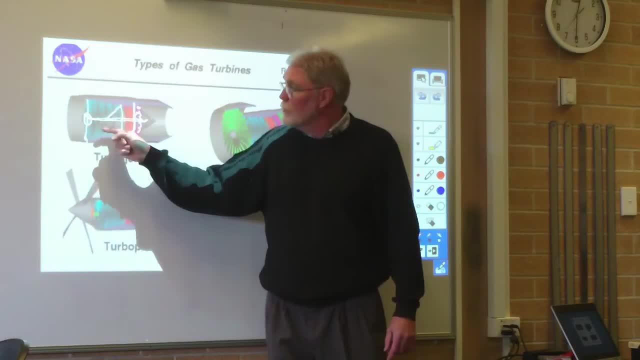 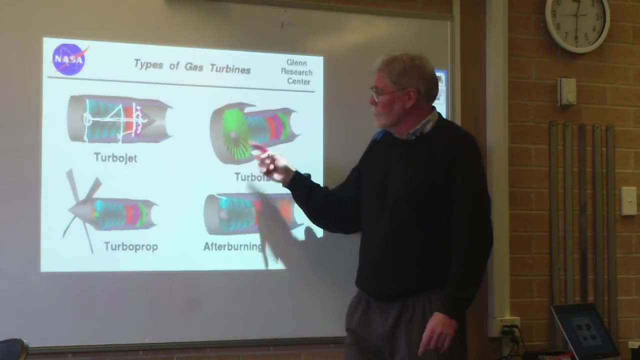 there was a drive shaft coming back through the front here that drives the fan. Well, if you kept the drive shaft going until it's stuck out the front, you can put a prop on the end of that. And that's exactly what these two guys do Now. you don't want it. 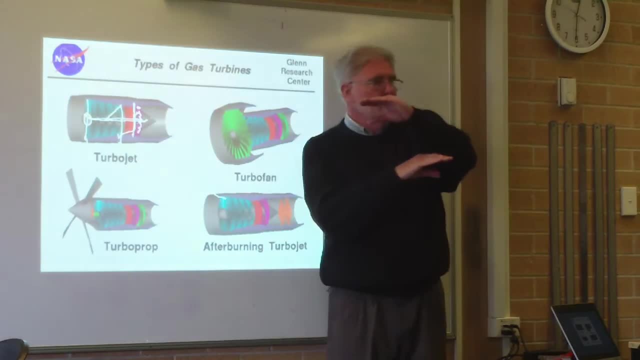 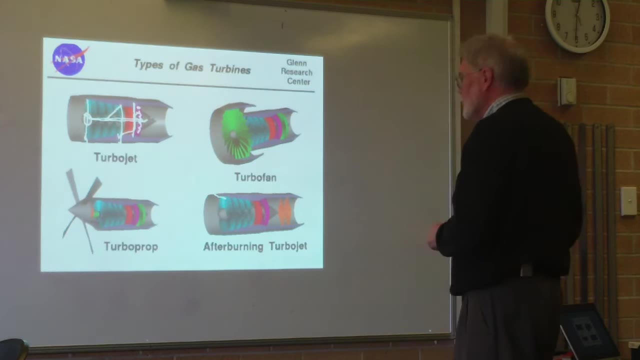 directly in front of the airflow. so sometimes these guys have got a big difference And I'll show you a slide in a moment where they're different. So that's the turbo prop and the turbo fan. You're actually running something else out the front of the jet. Let's get rid. 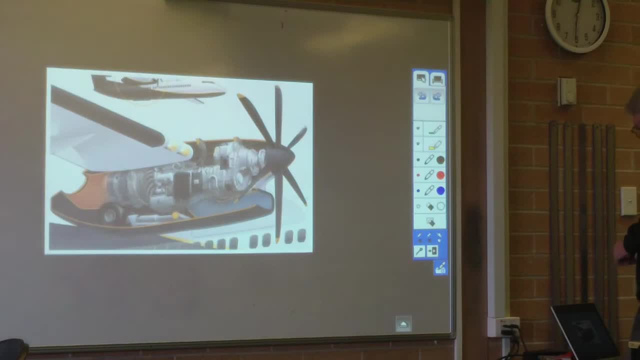 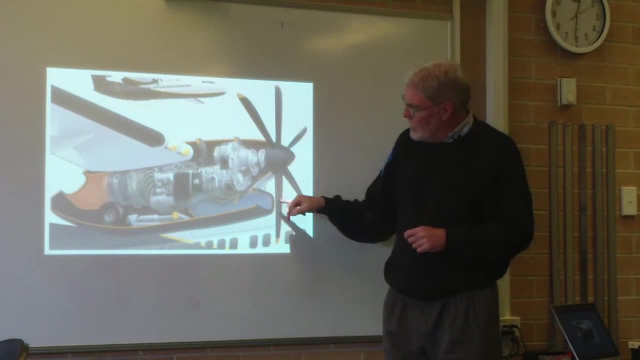 of that. Here's your turbo prop And the little bit more information here. to start with is, let me show you how that works. Big air intake here. that isn't like the other one, which is like a Ventura tube coming in sucking the air in. This one's just dragging the air. 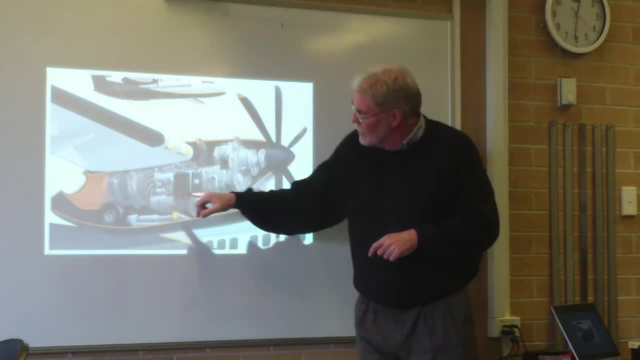 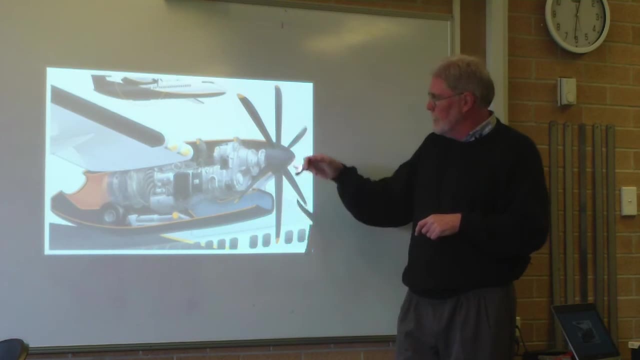 underneath the prop And as it comes into the jet engine element, which is here, the jet engine shaft is coming through and driving a gearbox which drives the propeller at the top end, And you can see there's a fair few propellers on this guy to get it going Now. 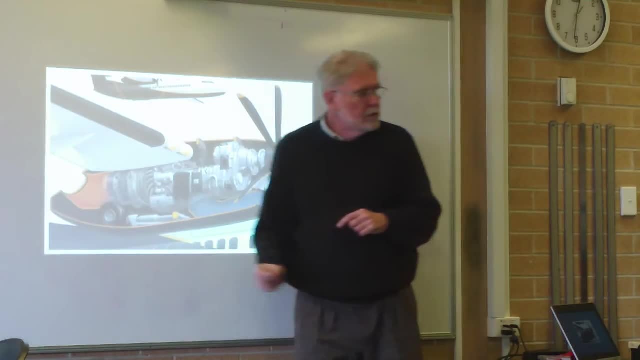 the jet itself, then, is assisting out the back. So there's a couple of things that you can do here. You can put the propeller on the jet engine, and if you're using a jet engine, you can put the propeller on the jet engine. 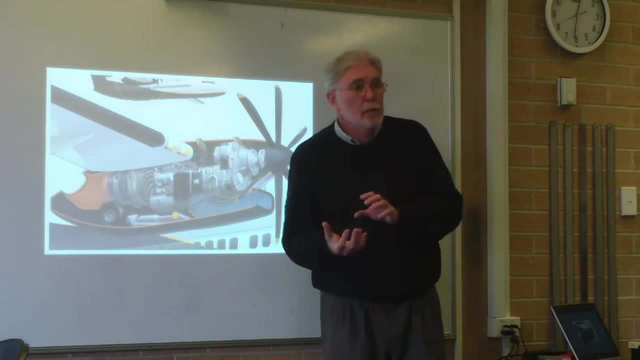 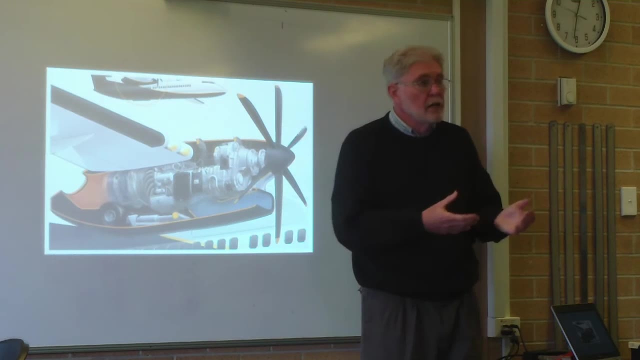 And this is the combination. You're getting the propeller to run off a jet engine because it's simpler. Simpler means less parts. Less parts means less weight. This means weights means more efficiency. So jet engines are actually quite good engines. Now we'll talk. 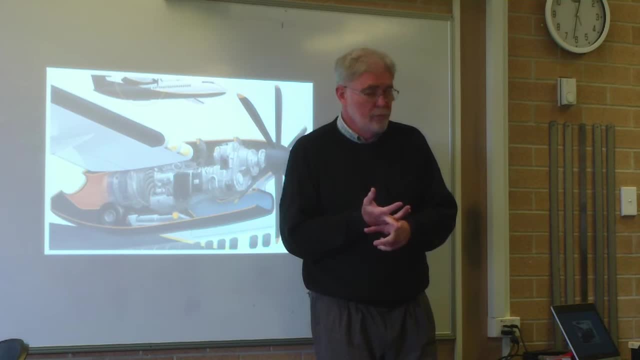 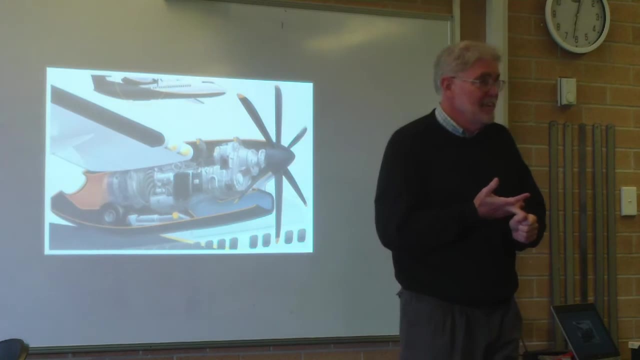 about something. and then you say, well, why don't we use jet engines for motor vehicles? If you think it through for a bit, you can see that one of the things you've got a problem with is heat. Jet engines run at much, much higher temperatures than your average jet. 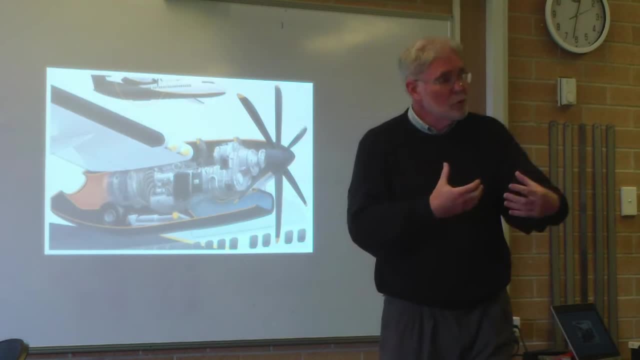 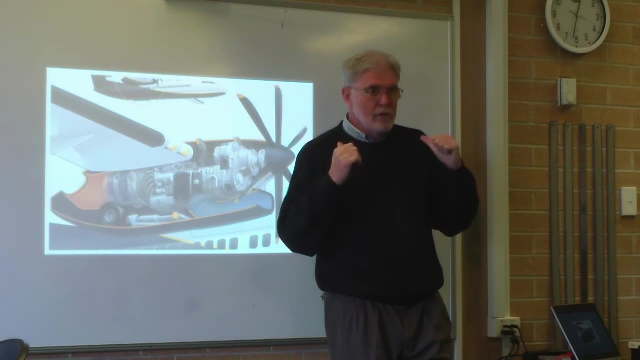 engine. So your average car engine with a radiator is within a range that's reasonably controllable. But if you put a jet engine onto a motor vehicle and you shove the jet exhaust out the back, the temperature of the air coming out the back would probably melt. the tarmac as you drove along. So you really don't want to do that. Or you've got to mount the jet engine really high so that doesn't happen. and then you've got all these problems of weight on the top and when you go around corners you're tipping the car. 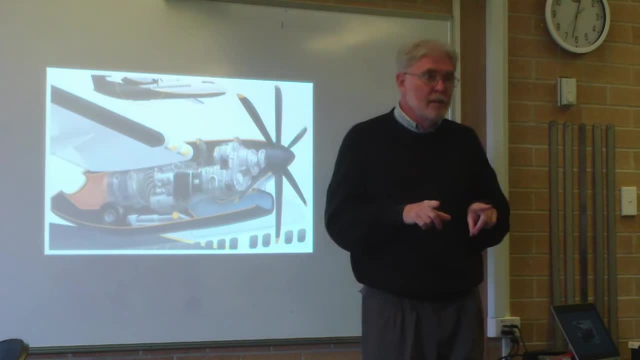 So fundamentally, a jet on a car is a dumb idea. You don't need that speed anyway, but it's a very efficient engine. Now there have been some attempts to put small jet engines into a motor vehicle and they haven't been particularly 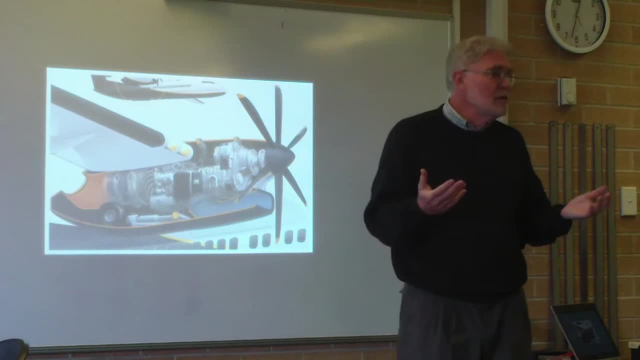 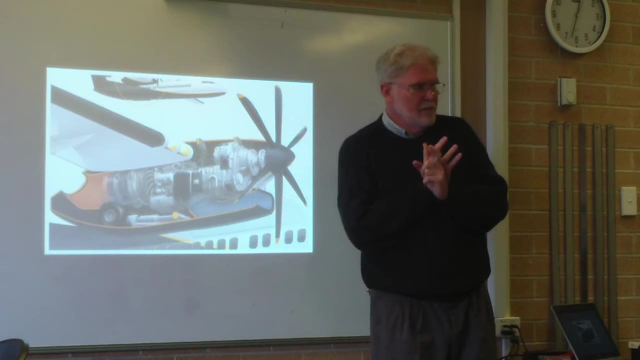 well received. to be honest, They just don't seem to be needed when there's just as much out of the efficiency of others. So I've just mentioned that jet engines are really efficient. Well, they're not. They're not as efficient as a motor vehicle. 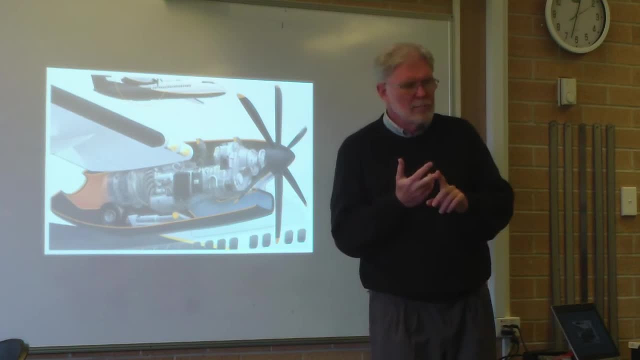 engine into a motor vehicle. They're not as efficient as a motor vehicle engine into a motor vehicle in terms of what you get out of them- and I'll explain why in a moment. It's mainly the heat- But they are in terms of their weight and the number of moving parts. 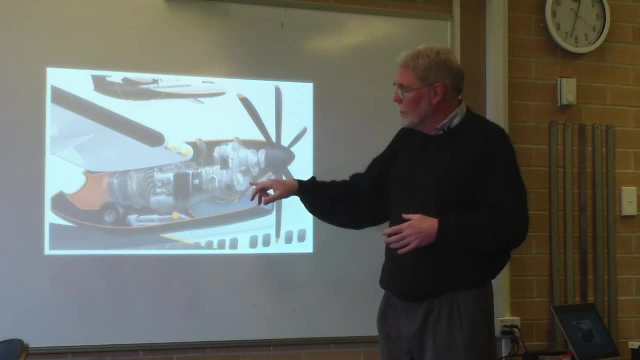 So they're a simpler concept. There's not much going on. It might look complicated, but compared to the Rolls-Royce Merlin engine, it's a lot simpler. The other thing about them is that it took a while, and I was going back to this. I was 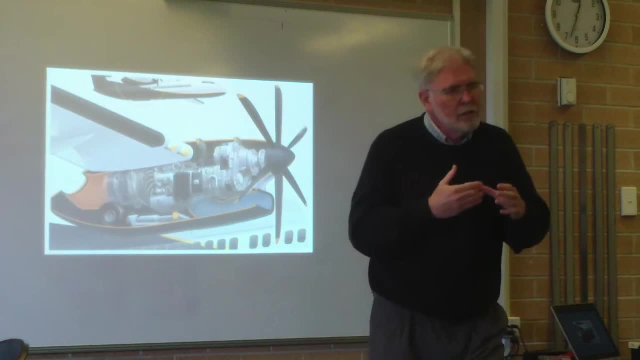 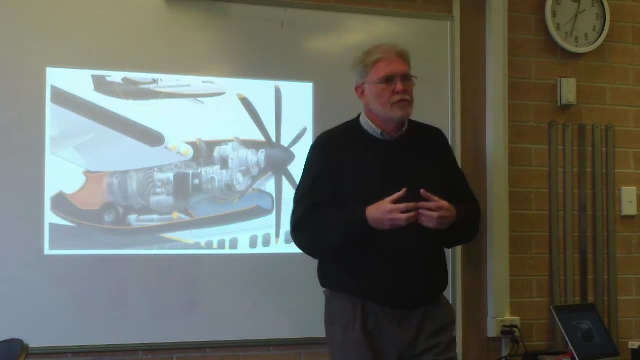 saying before about in the mid-30s, something else was needed to make a jet engine possible. The temperatures we're talking about generating are very, very hot. They're in the orders of around the 1400 degrees Fahrenheit. Now most metals, including steel, can be melted. 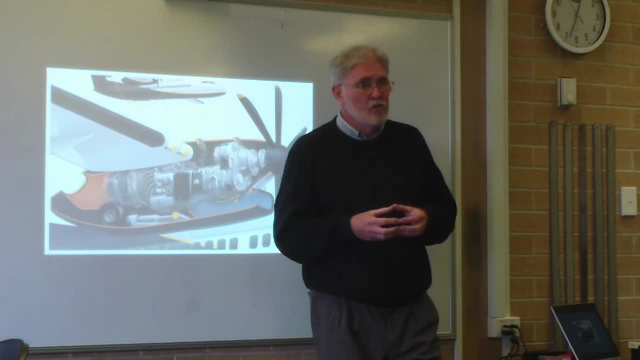 in those sorts of temperatures. So you're not going to want to build an engine that melts itself. That's not a very good engine. And the other thing is that if you can't contain the violence that's going on inside, you can have a catastrophic explosion as a result. And the very first few jet engines when they were turned on often did They just accelerated themselves to a point where it was runaway speed and they blew themselves up. So all the control mechanisms, the kind of metals you needed to have, were not available technologically until the 20s and 30s. And then they started to do some stuff with some. 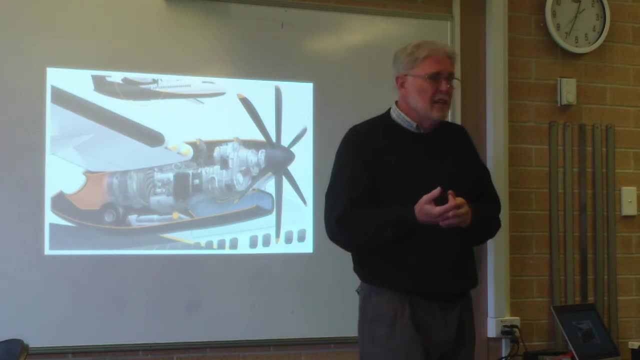 alloying high temperature alloys. now, the other thing about an engine that's running at the speeds that these things run at is that any tiny, any tiny imbalance and the engine is going to cause catastrophic problems at the end. the tip speeds for these rotors can be quite pronounced too to get the efficiency you need for these engines to compete with petrol engines. you have to run them at really high speeds, you have to run them at really high temperatures, and both of those preclude them from being used on the ground as a normal means of transportation, but in the air they come into. 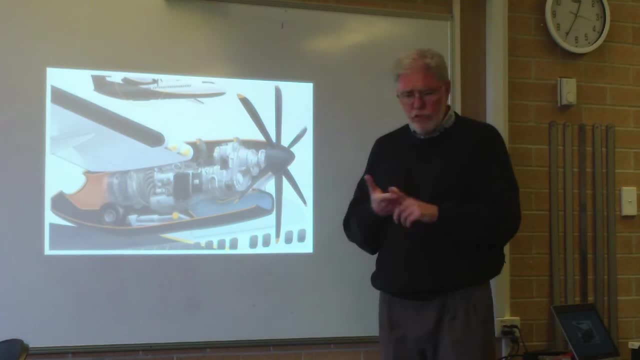 their own, as we'll see in a minute. okay, so jet engines: simple, not very efficient in terms of the way in which they generate. um, what energy is being used? because there's a lot of losses, but you can utilize those losses to help you with your driving by the heat coming out the back. 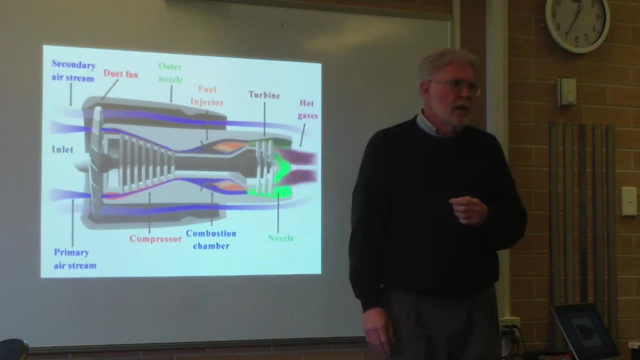 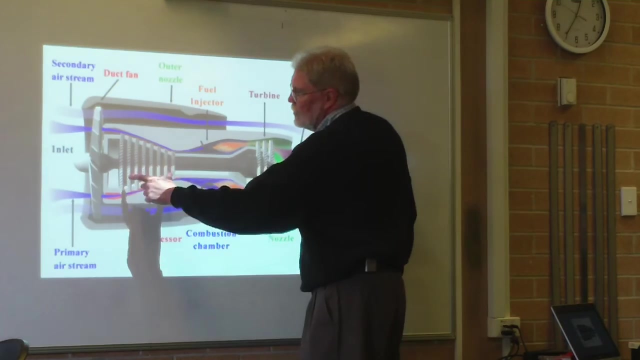 this is the one that um currently used on most of the large intercontinental aircraft. this is called a high bypass fan turbo fan engine. in this particular model, what you've got is the original jet engine situation. so you've got the three compartments, you've got your compressor section. 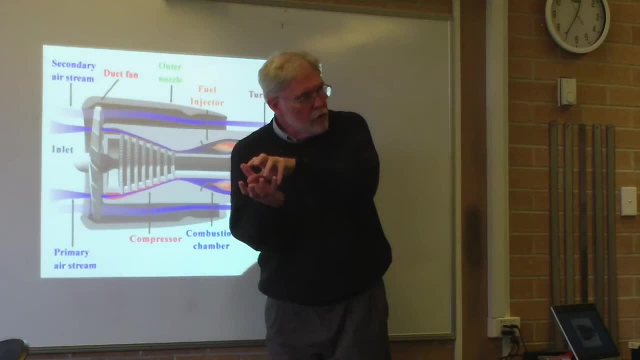 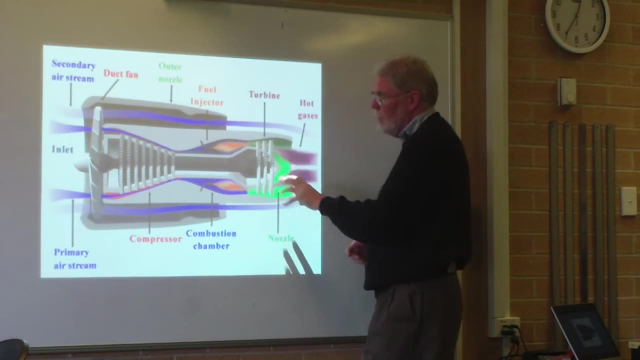 at the front, with the blades getting smaller as it goes, squeezing the air in tighter spot. so the air is accelerating and heating up. at the same time it's coming through into a burning area where you're pouring a tiny little bit of fuel in igniting the fuel, which further excites the air. 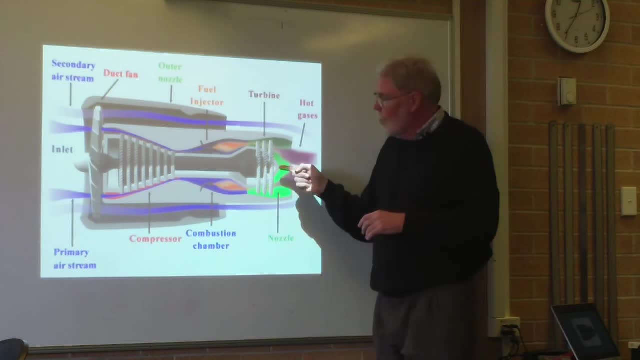 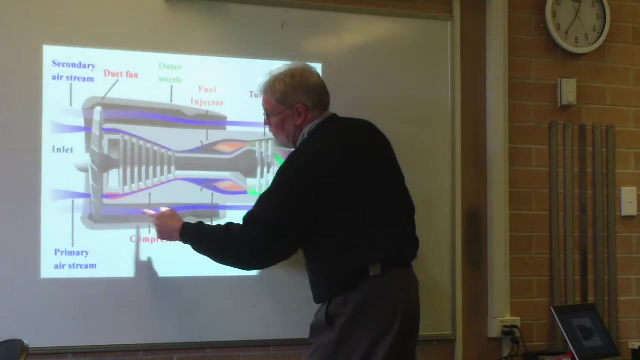 which then pushes on a turbine set at the back, all driving a drive shaft connected through to a large fan at the front, in front of the compressor. it's called a high bypass engine, because now what you're doing is getting some additional airflow around the engine, which does two things helps. 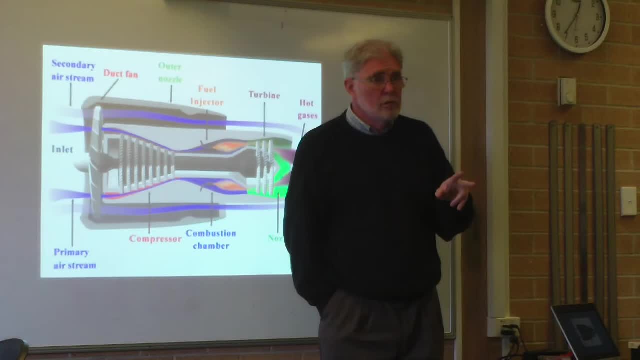 with keeping it cool, helps with keeping it cool and also, uniquely, quietens the engine now, because you now have a moving air barrier between the sound of the jet and you can use these jets in. well, now you can, they're using them more and more to extend the range of times that you can use on. airports because one of the complaints about jet engines is they're extremely noisy when they're taking off. but these high bypass fan jet engines have quietened them that down. some of them are so quiet that sometimes they compared to the old-fashioned jets. you know you probably wouldn't even know they were running from a distance of a kilometer because they're. 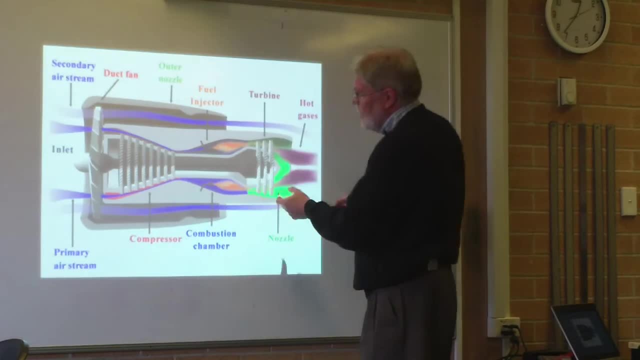 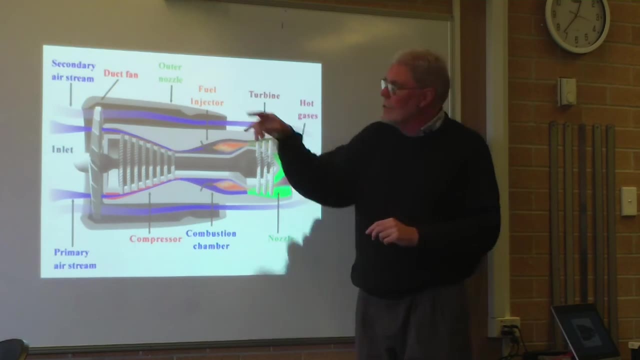 that quiet. so this gives you more efficiency. when you just have the jet engine and no propeller at the front, the only only thrust is coming from what you get at the back. now you're getting this additional thrust from around it, which is cooling and helping keep it quiet at the same time. so 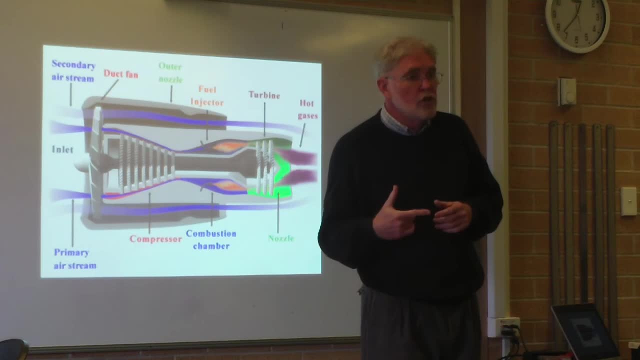 these jet engines now about thirty forty percent more efficient than the original jets, which makes them commercially economic and makes the idea of putting a lot more people into commercial aircraft more. it's more reasonable for companies to do that. it's one of the reasons why there's pretty much an expansion now in travel by air, because these things work so efficiently. 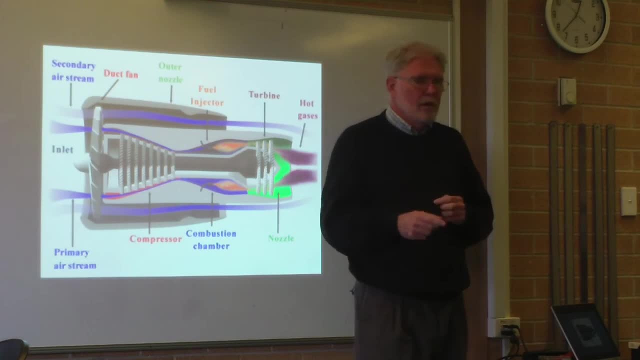 for you in that now, efficiency I've mentioned about five times. I still tell you that the in terms of, in terms of how your heat loss and where it all goes, a jet engine is not very efficient. the most efficient engines tend to be electric engines. electric motors will give you a better 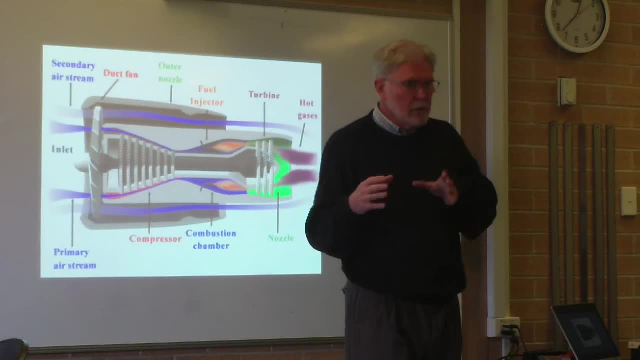 return. you can get up to 80 to 90 percent sort of things from an electric motor. you're only getting about 30 to 40 percent efficiency out of these aircraft engines. that's not real cool. petrol engines somewhere in the range of 60 to 70 or so percent, because there's still heat losses. but you 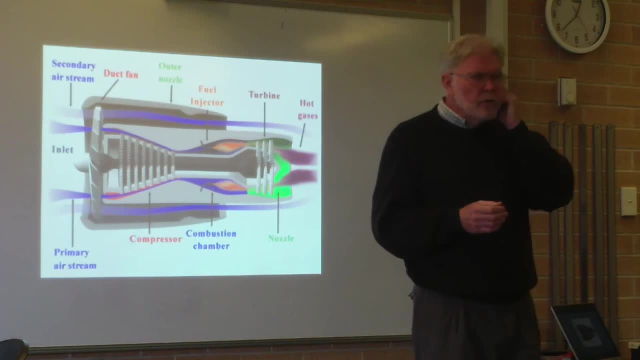 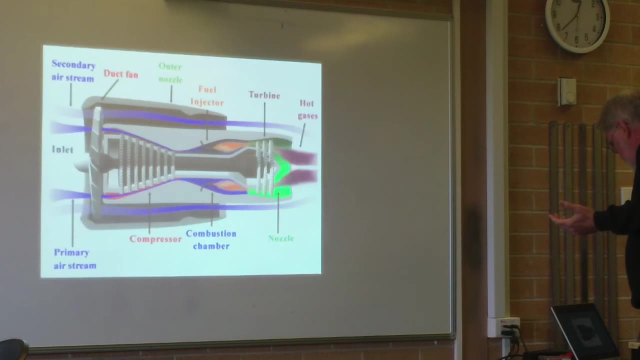 you've got that control. so now you start to think, well, if there's that not very efficient, why would we use them? why wouldn't? of course, we've got two things: we can get out of the engine and we can get out of them. let's go back the other way. this is probably the key thing now. it's an interesting question to ask: what is the difference between air down, close to the ground, and air up high density? density, yeah, because the column of air above you is less, so you are going to lose the amount of air as you go up, which means that grabbing the air and pulling it, pulling yourself through it with a propeller, gets less and less efficient as you go higher. so you tend to find that certain aircraft have a limit. helicopters, for example, rely heavily on there being a large mass of air to hold, lift up just quickly. there's another thing I remember to mention, meant to mention this. there's a particular jet engine called a turbo. 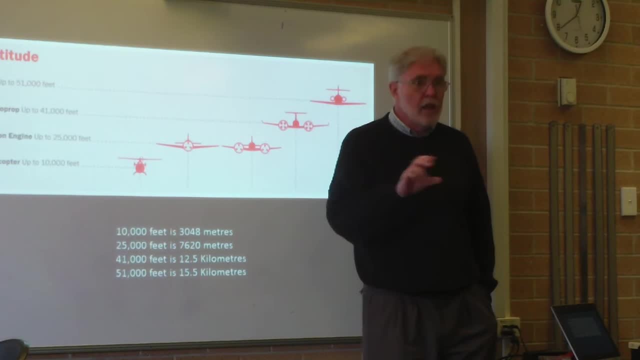 shaft engine. the turbo shaft engine is a jet engine that doesn't have a propeller out the front, it doesn't have a fan out the front, doesn't use the jet as its main form of propulsion, but drives a motor, drives a gearbox or a shaft. it's the kind of engine that, in fact, 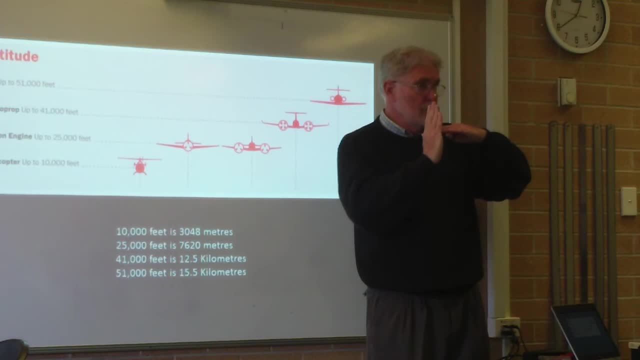 the shaft can often be at 90 degrees to the engine. it's the kind of engine that gets used for auxiliary power on some planes and there's a tiny little. sometimes you see on big, say, 747s, you've got that little jet at the back of the tail. 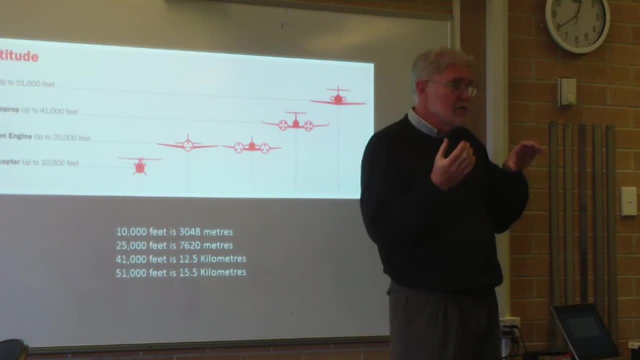 hold it back. it's auxiliary jet. it's really just there to run things like air conditioning and generate power, because you can't- you can't- plug your aircraft into the local power socket when you take off. so whatever you go up with, you've got to take with you. so all the lights. 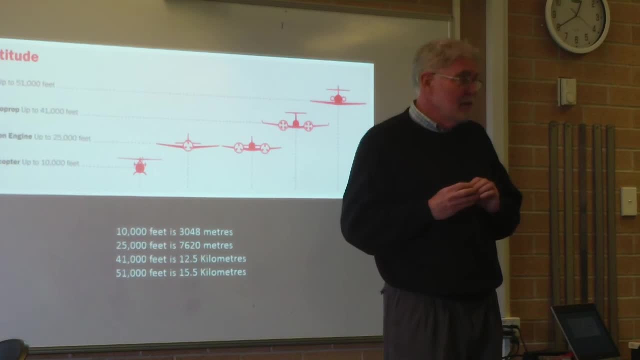 and all the electronics that you're running have to go with you, and if you're going to fly for hours, batteries are not a good idea, so you better take a generator with you. so they use one of them as an auxiliary generator and they still use a jet engine because you've got jet fuel on board. you're not going to have. a different set and it works really efficiently at the high altitudes. not that's petrol engines, when you get up high, rely on air. they burn with air. so if you're getting less and less air, you're not going to get the most out of your petrol engine. at high altitude it'll start to starve. of air and you won't get the engine to work. that's possibly too right. so turbo shaft engines get used to, or, for turning right angles, to run propellers on helicopters. but you're still limited to the amount of distance. now I've converted some of it to see how far up you go. so 10 000 feet is about. 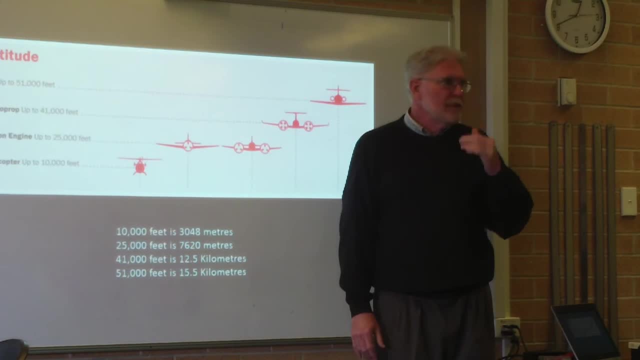 three kilometers. now you might think three kilometers is not very far when you look at it on ground, but when you start talking about 51 000 feet or 15 kilometers, you're now at the height of Mount Everest. you're on oxygen when you're up that far, um spy planes, you know Blackbird. things like that fly at around 60 to 65 000 feet, so they'll go up to around 17 kilometers, and which puts them at the bottom of the troposphere, going into the stratosphere. and the troposphere is really that area where you um, there's oxygen in the air enough. yeah, you don't want to go any higher. 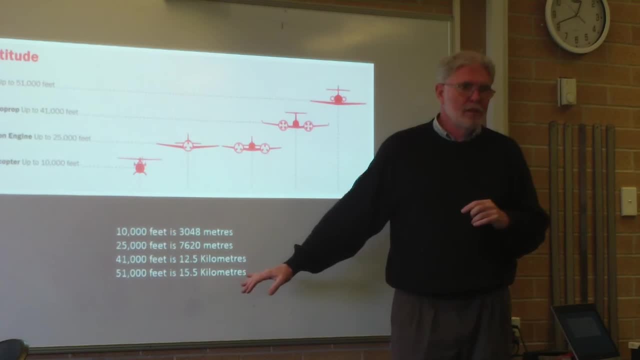 you're on oxygen by the time you get to this place anyway, because you're just not being able to breathe. but there have been people who should know- probably if you watch that movie Everest- who have walked um. they have to acclimatize to do it, but it's possible so you can breathe at these levels. but once you go a bit further up, there's no oxygen to breathe, so you can't burn it because it's not going to be there to burn, so you can't run your planes. the other thing is, of course, propeller engines, again like that, are going to rely on dragging the air. so if the air is getting lighter, the higher. 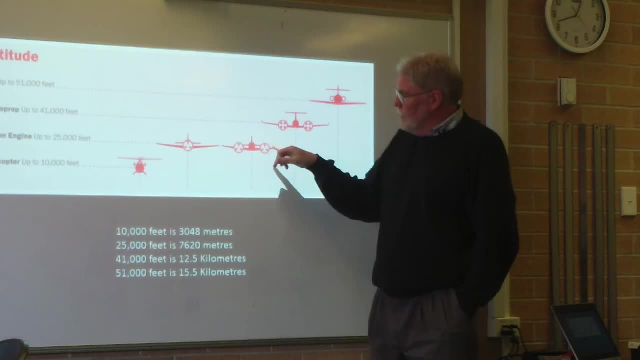 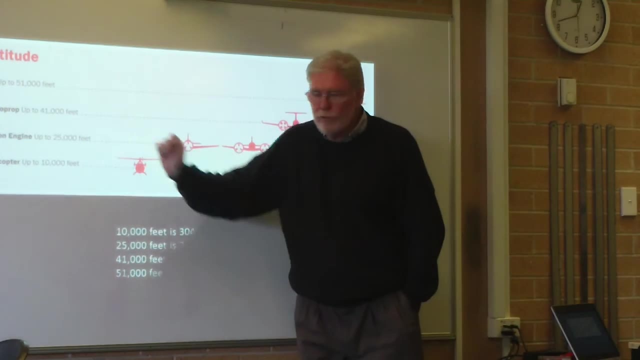 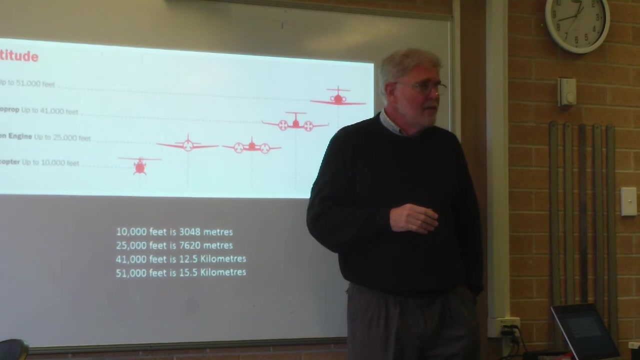 you go. these, as I said, are more efficient, so why don't we use them more well? we do short haul all the way with 25 000 feet, particularly in Europe, particularly in America- and maybe you could consider New Zealand and other places like that- there's mountains in the road. 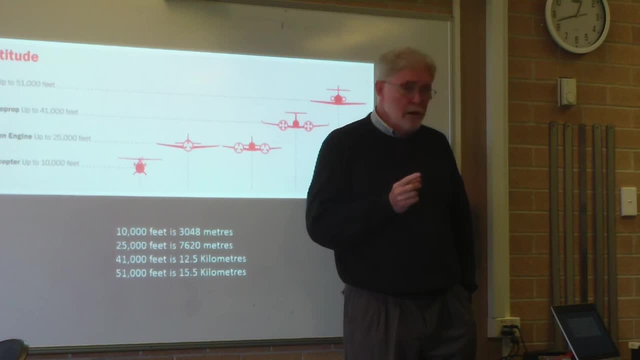 so if you want to fly straight lines between places, you better hope there's no mountains between you and them. often that's what causes problems with aircraft running into mountain sites and lots of crashes in the 30s and 40s because they couldn't see it, because they didn't. 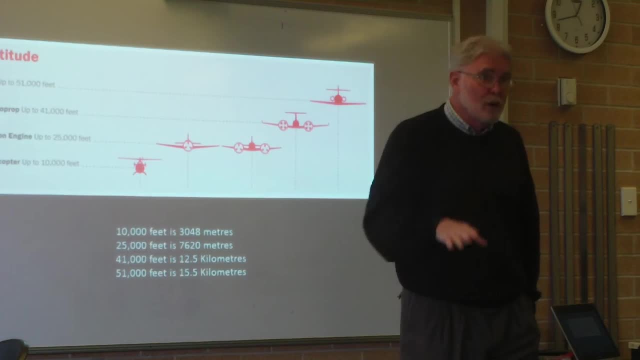 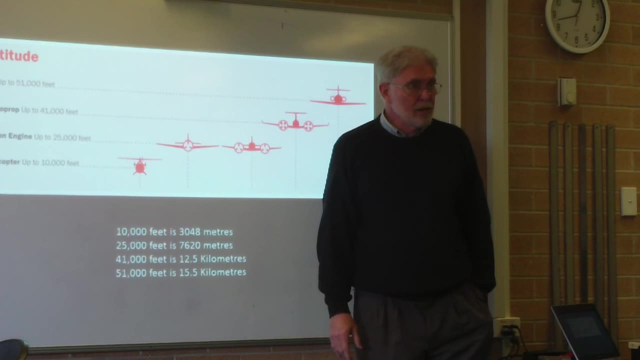 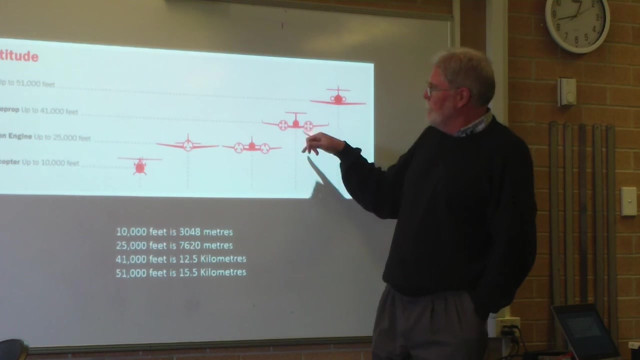 have the sort of technology to be allowed to see things in the fog and rain and stuff like that or at night time. so you're you're problematic with aircraft flying down low. there's things you can run into: not many houses, but plenty of plenty of um mountains, turbo props. this is the one where you're using the jet. 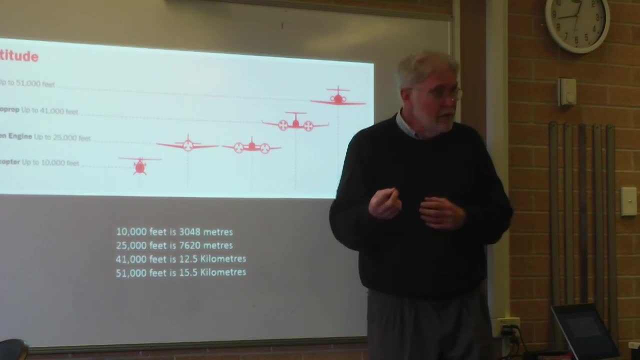 the air. you're running a propeller to drive it, so it's got a limit to how far it can go. and the last one, of course, is Jets right at the top. now there's a reason for why Jets get used at the top rather than generally speaking. these are short haul, pretty much where you can see where. you're going because you don't want to run into anything. even at 41 000 feet you still got some mountains around, particularly in Europe, and that are at those sorts of outages, um, but you're still more efficient because you can fly higher once you go up a little bit too. 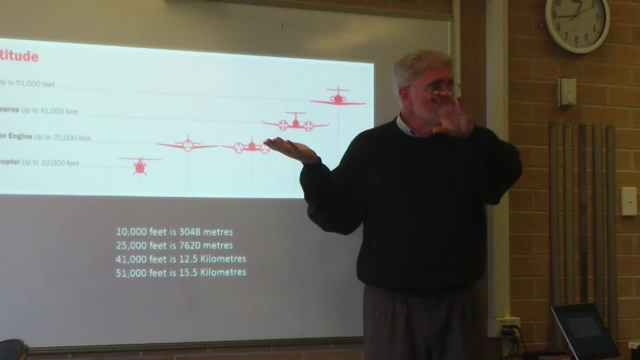 you start to pick up on movements of air, mass movements of air at certain levels, jet streams, the way in which the air cycles down low, uh, creates our wind down low in turbulence, in our storms, and all our clouds tend to be in this lower section up to around the 41 000. feet sort of area. so once you get up here you can fly above most storms. now you won't fly above something like a hurricane, because the air being dragged into the hurricane is coming from the troposphere. it's been pulled down. it's one of the generations of what gets cold air coming down. it keeps that thing running. so once a hurricane, a cyclone gets large enough, it starts to drag air from up up higher, cycles the air into the whole process. so you know you want to fly around hurricanes and cyclones but your normal every Saturday afternoon sort of, you know, like hot. summer day thunderstorm, this sort of range. here you can avoid them. but once you start going higher than this you haven't got enough air to use a propeller. you're stuck with the jet. but the thing is that poor efficiency down low once you get high the jet. 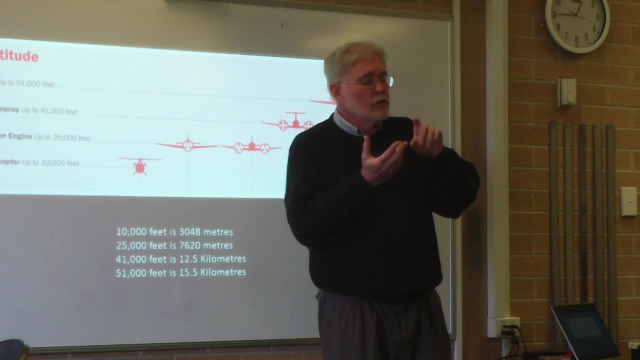 engines now come into their own, because now you're flying at altitudes where you have less problems with the air in front of you. you know there's less drag as a result of the air in front of you, you are able to travel in straight lines without having to avoid things on the way. 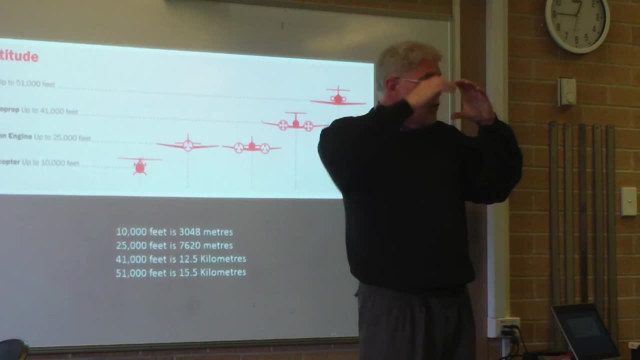 you get the assistance of having these low troposphere jet stream air movements that are moving in bulk above the cycles of normal day down below. so you get over all of that stuff and you get. the compensation for the lack of efficiency in the engine is now in the fact that you can travel at 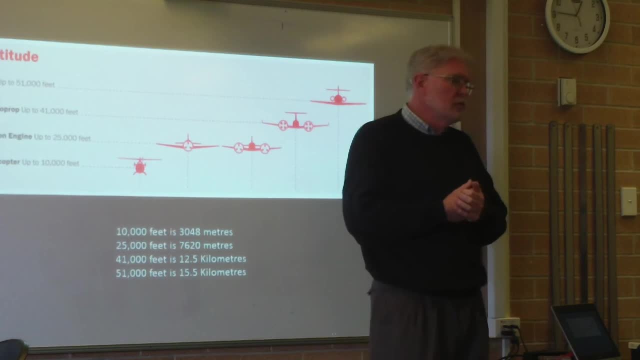 high altitude, all right. what was the problem about high altitude flight that stopped it from happening? in the flight oxygen, yes, you now have to have a pressurized cylinder and you have to have air being used in a different way for the people involved so you feel comfortable in the aircraft at those. 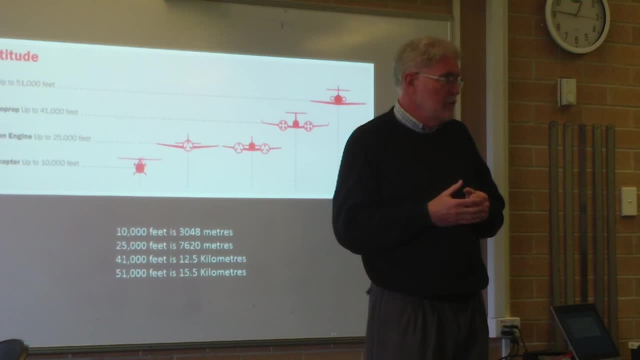 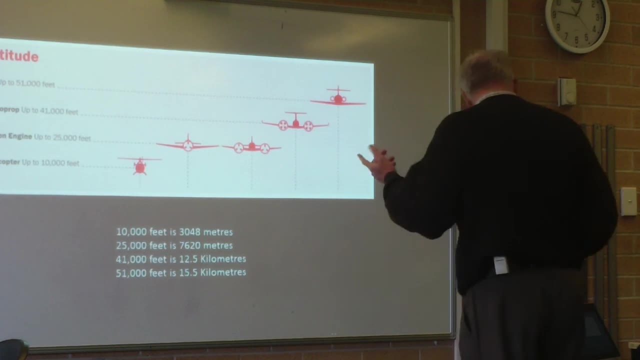 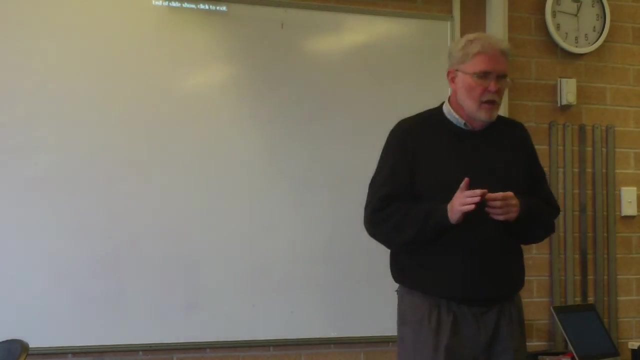 altitudes. you also have issues about rapid decompression. so if you have a problem with a hole in the engine, it always happens because it's going to be anyway, that's. that's pretty much the end of the day in that section. I've got some notes on the motors for you to take so you can look through that's.